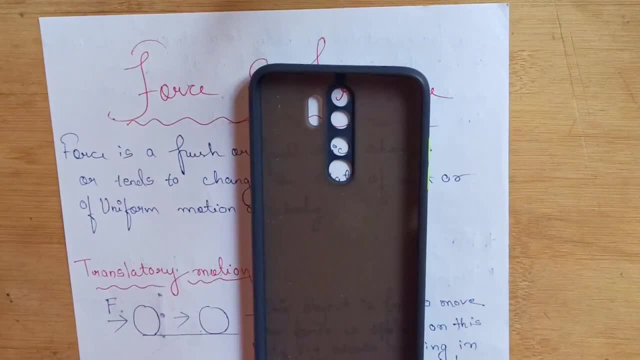 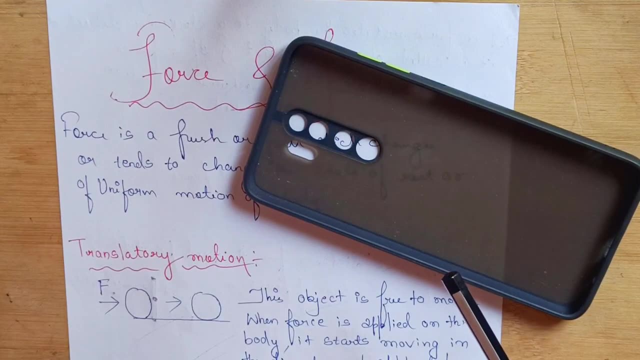 I gave it force. So what happened? because of force, It was in rest. How was it? It was in rest. Now, because of giving force, it came in motion. Motion means there is movement in it. So what is force? children? 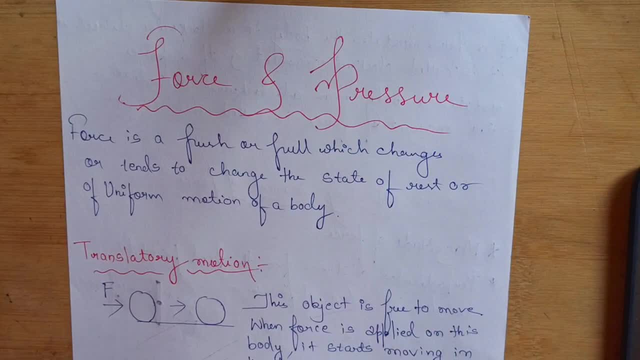 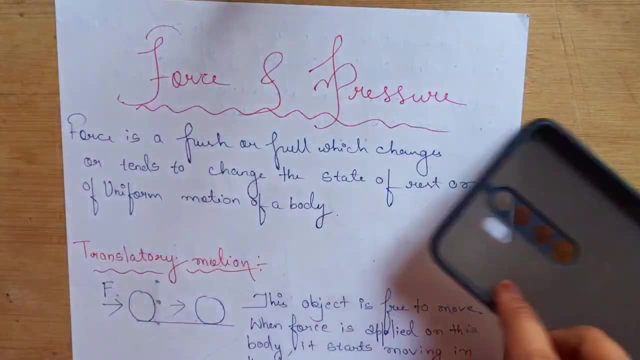 Force is a type of push and pull Because of which there are a lot of changes in the body. If a body is in rest, then if I give it force, then it comes in motion. If a body is in motion, like a ball is coming. 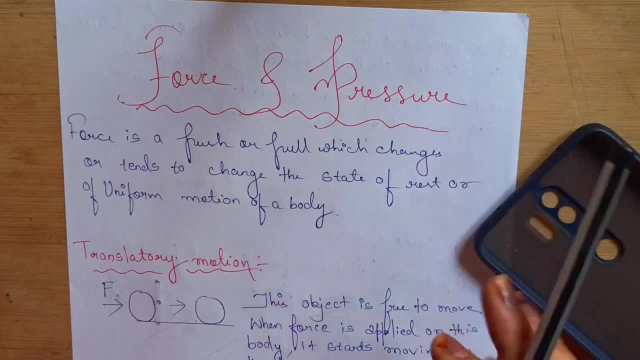 The filter is ready to catch it. So the ball was in motion. The filter will give it force, So it will stop the ball in its hand. So because of force, the object which was in rest, It can do it in motion. 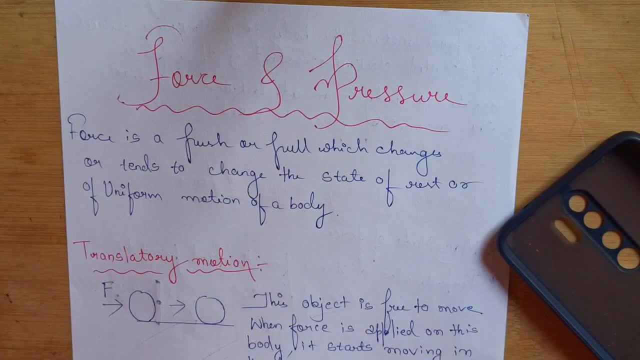 The one which was in motion. it can do it in rest. Many more things can be done. If we give force, then we can change the shape and size of the object. If I give force in it, then its shape and size can change. 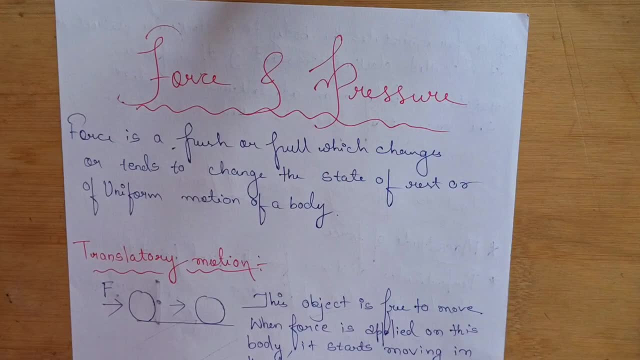 Definitely it is also breaking, Isn't it? So force is a type of push and pull children, Because of which the state of rest or motion of the body has changed. Many changes are made in the body. Its shape and size changes a lot. 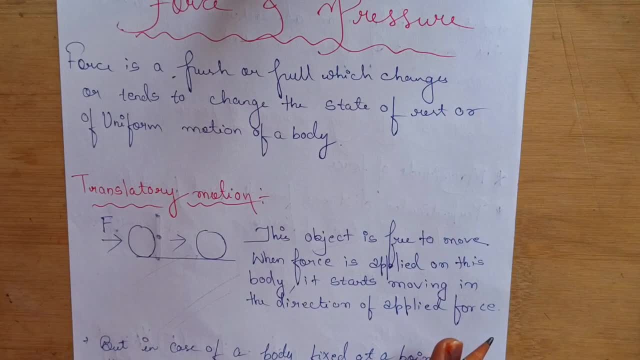 Now here is a term That is translatory motion. What do we call it Translatory motion? So this motion, you will read it in higher classes also. It is more in class 10.. It is more in 9 also. 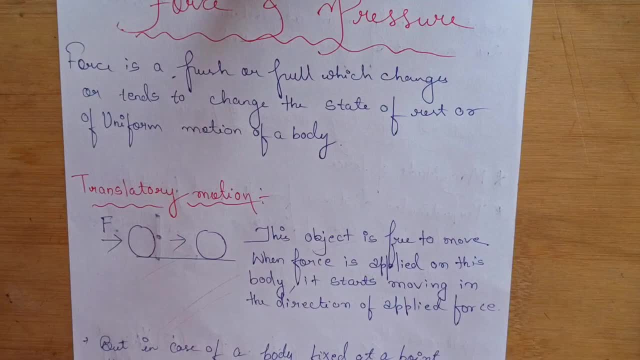 But it is more in 10.. Ok, So what is translatory motion As children? there is an object here And this object is free. This object is not attached from anywhere. That it will stop after going half way. There is nothing like that. 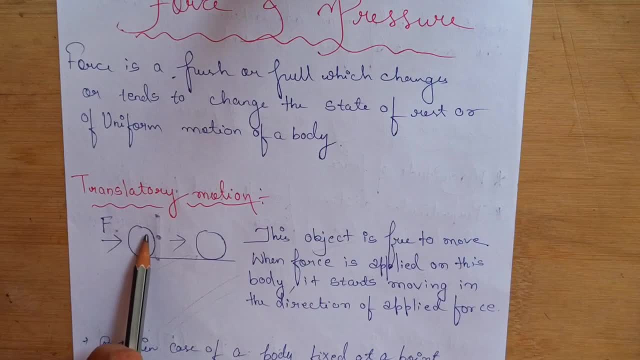 This body is free to move. Ok, So this is an object which I have shown in round shape And here I have written F by doing arrow. That means here it is talking about force, As there was an object, here It is a free object. 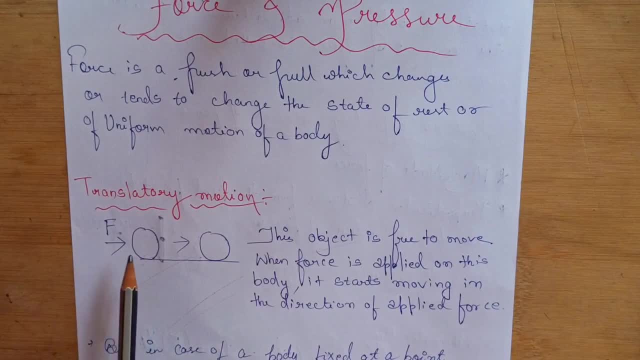 Free to move. I have given it some force When I have given it some force. So due to that force that body will move a little forward. And here that body is moving on a straight line. All the particles of the body, 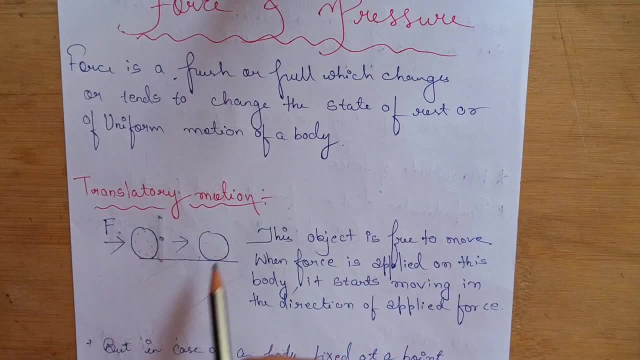 Like in this body, This much, this much, this much, All the particles, They are covering equal distance here, Due to force, The direction of all is the same In the direction in which we have applied force, Like we have applied force. 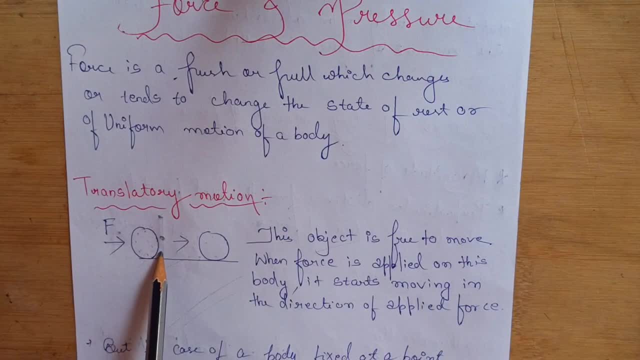 In the same direction, Like here. in this direction we have applied force, So this object is also moving in the same direction. This object is free to move, The object which I have taken here, That is free to move. So when force is applied on this body, 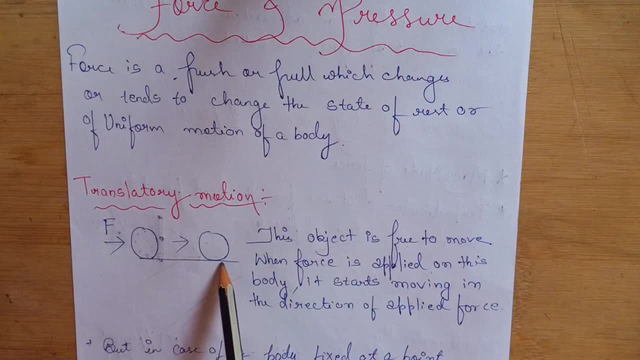 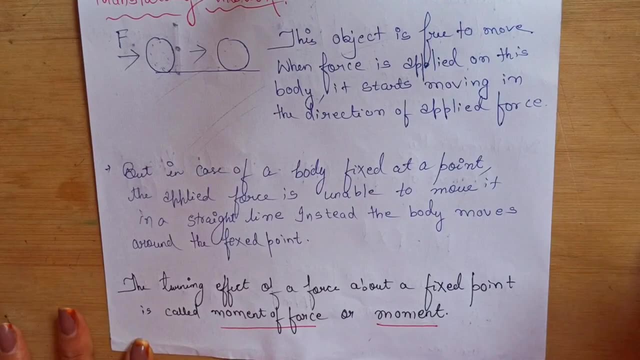 When we apply force in this body, So this body will move in the same direction, In the direction in which we are applying force. Ok, So this type of motion, So children, if we get to see this type of motion, Then we call it translatory motion. 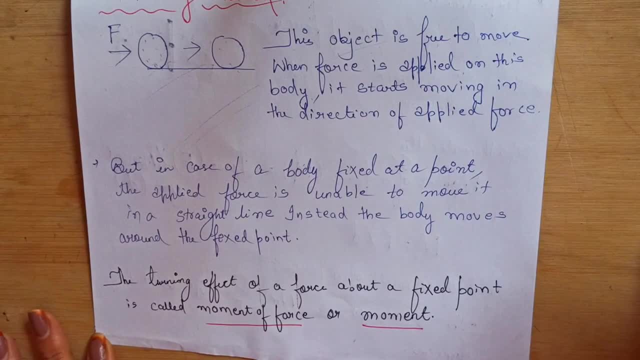 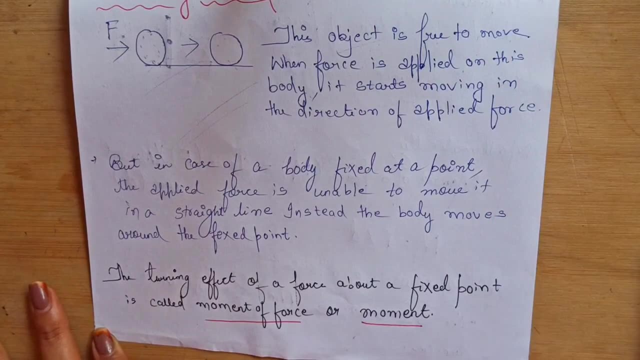 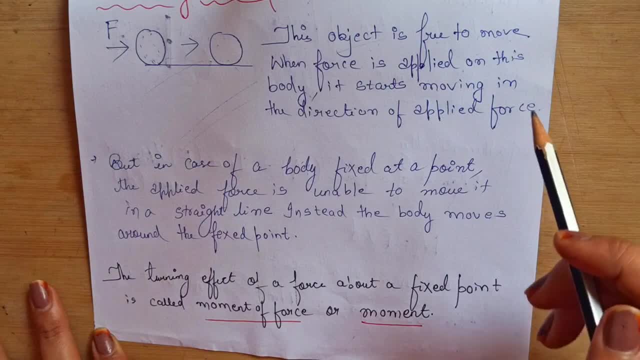 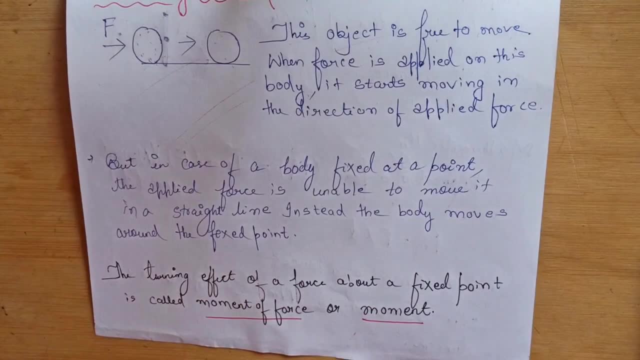 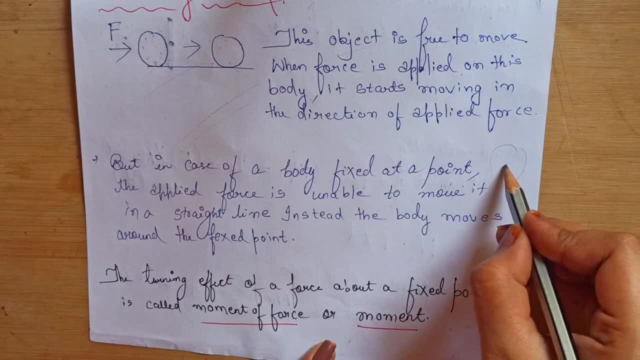 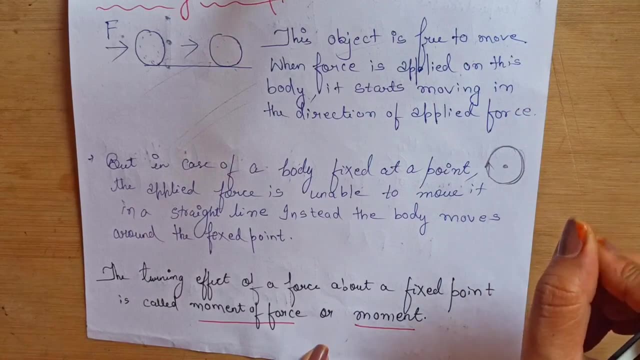 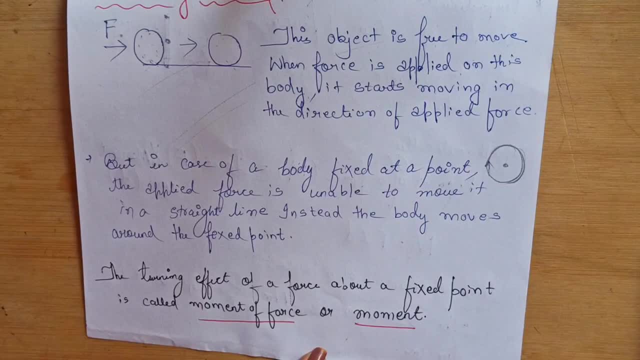 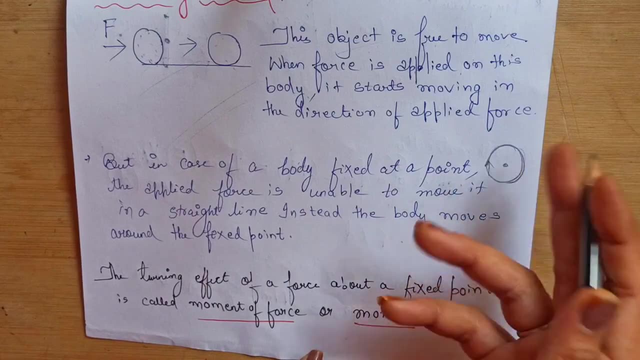 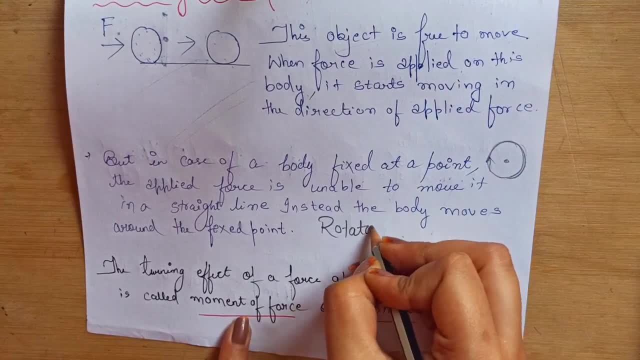 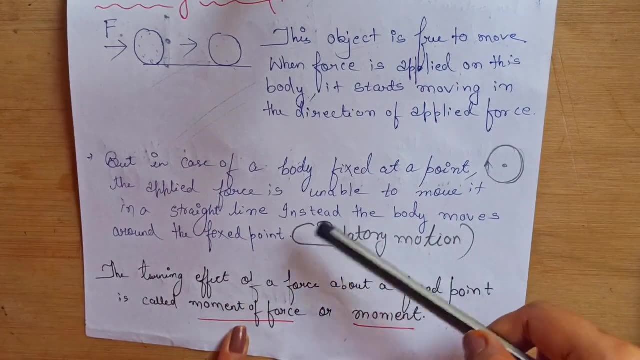 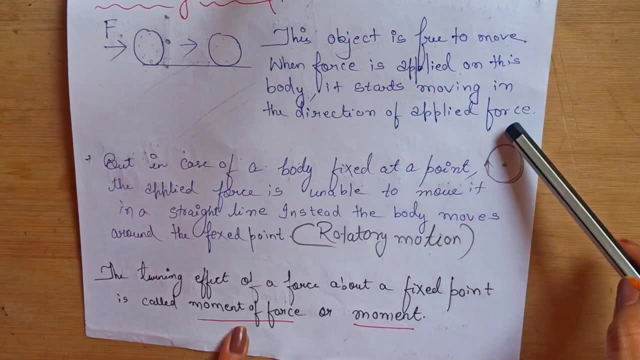 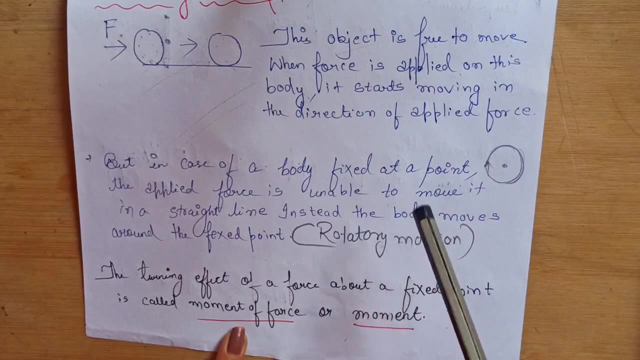 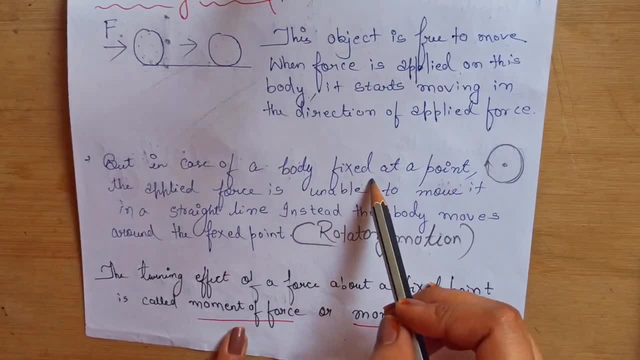 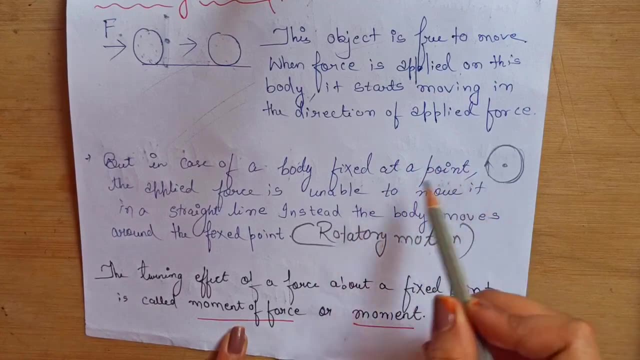 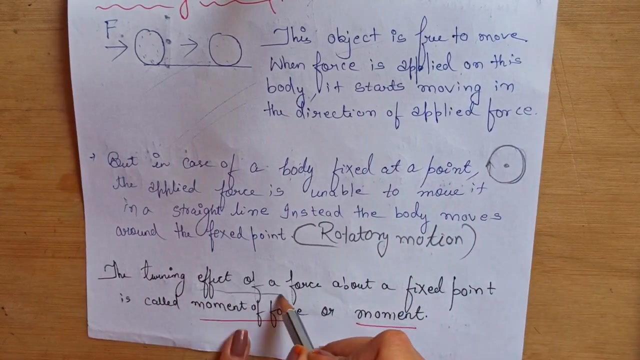 motion that is given. the object was fixed in one point. when we gave force it did not go on a straight line. it started to rotate, So it turned. So because of force, a turning effect was produced. Because of the force the object rotated. that means the turning effect was produced because of the force. 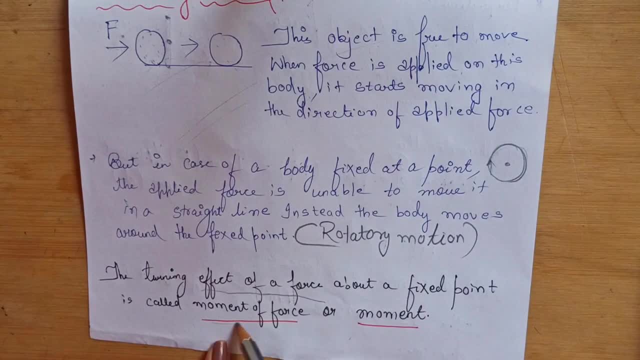 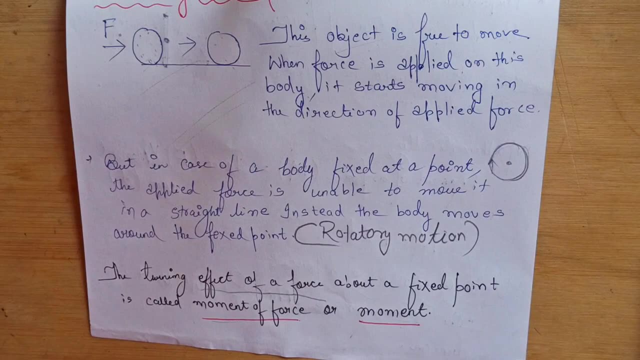 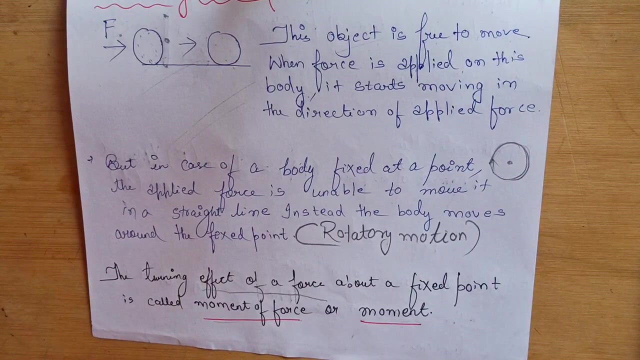 So if such a turning effect is being produced, then we will call it movement of force or just movement. Okay, movement, kids movement, okay. So here about a fixed point, a turning effect is produced because of force, Then we call it moved of force or just movement. simply, what do we call that? We will call it movement. 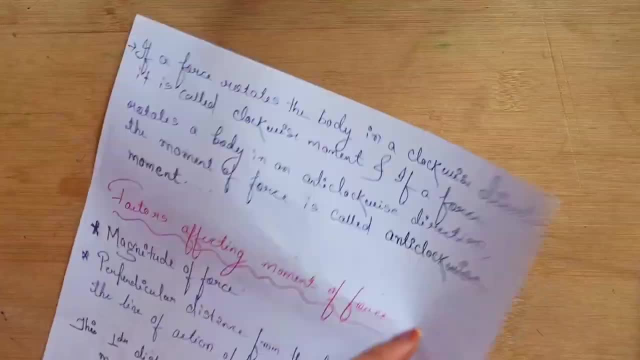 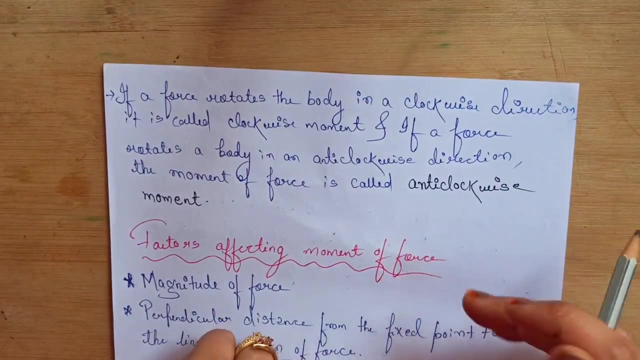 what will we say? We will call it movement. Okay, what will we say? We will call it movement. Now I give you the example of this. Take a door, take a gate. Now you know that the gate is fixed in one way. 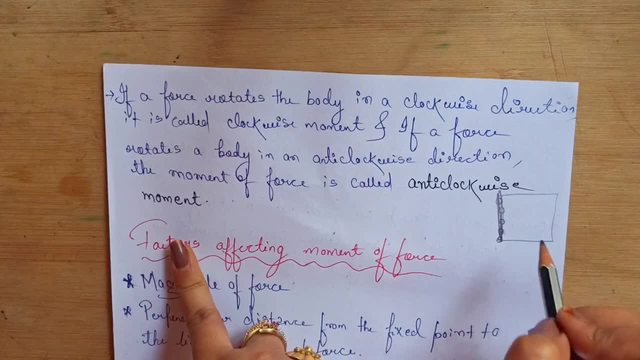 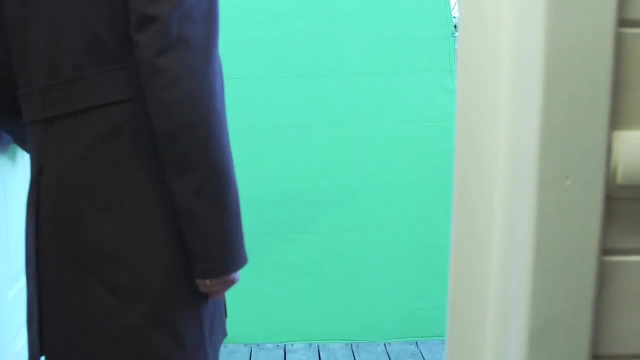 suppose that the gate is fixed from here. I am giving you the example of the rotatory motion. Now the gate is fixed from one side. Now you will give force in the gate. If you give force in this direction like this, Now tell me, Will the gate go straight in the direction of applied force or not? 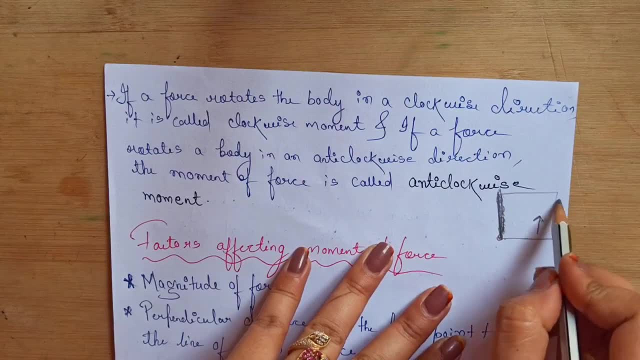 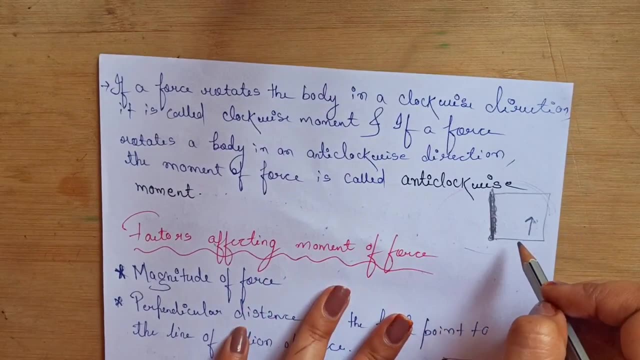 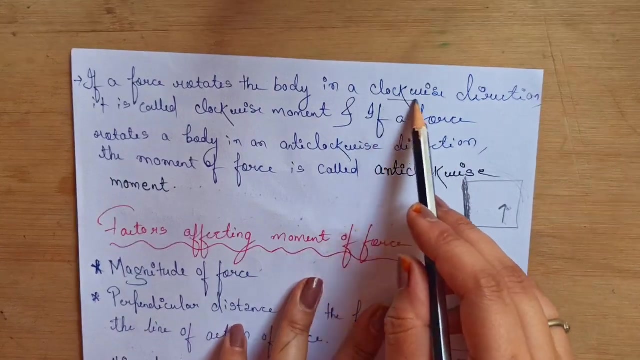 We call this hinge. It will move in this direction from both sides, From front to back, Because of the force we are giving. here the rotatory effect is produced. Turning effect is produced Because of the force we are giving If the body moves in the clockwise direction. 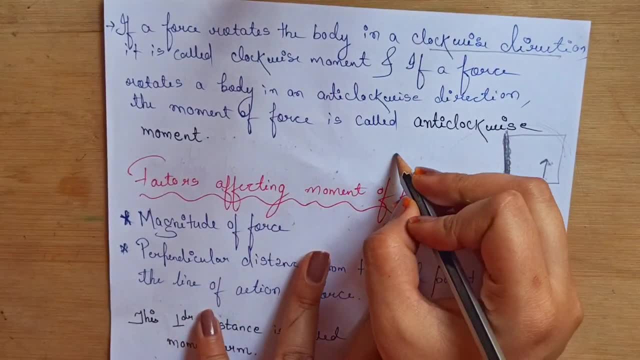 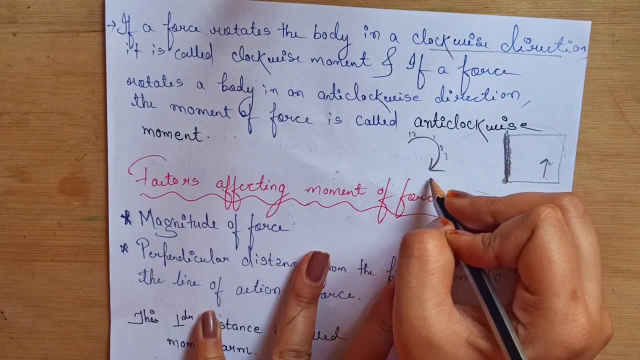 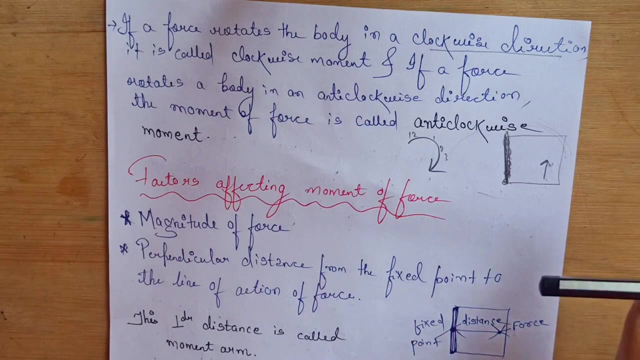 Clockwise direction means The way the clock works In this direction. 12,, 1,, 2,, 3. If the body is moving in this direction, For example, if you push the body and give force- Because of that force the body did not go on a straight line. 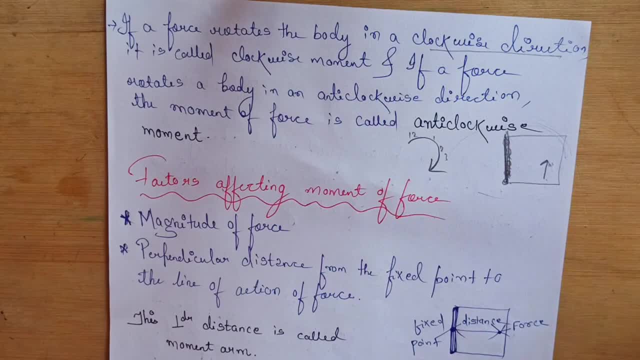 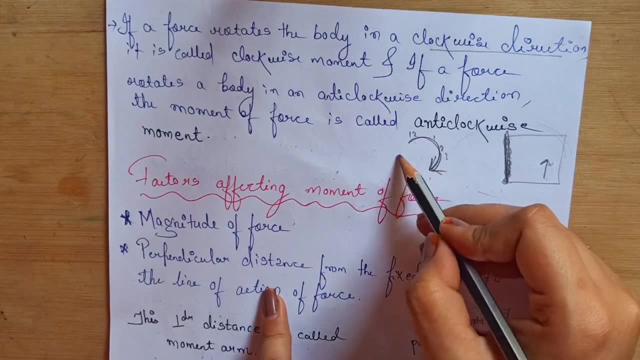 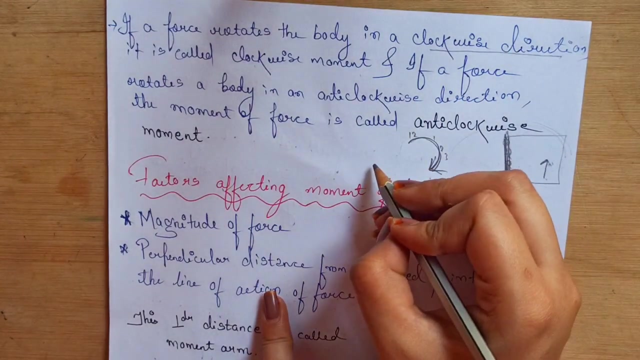 But Because of the force, the body is rotating in the clockwise direction. If the body rotates in this direction, So we call that movement clockwise movement. And if you give force Without going on a straight line, If the body is rotating in this direction Like this. If the body is rotating in this direction, 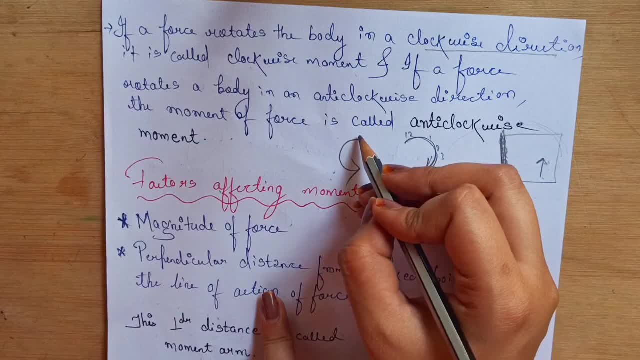 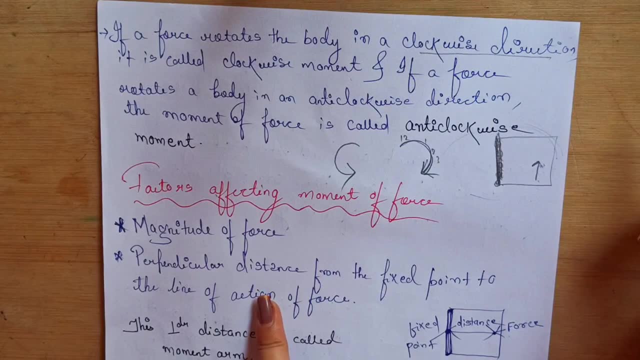 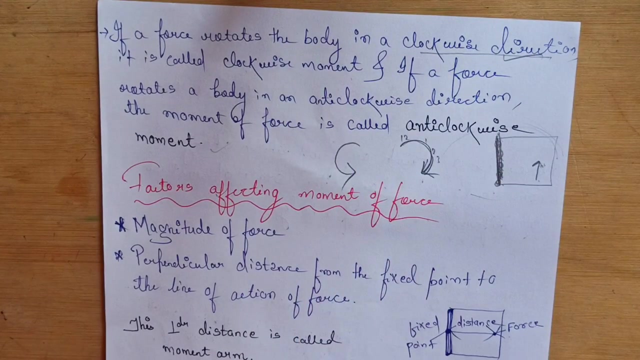 Then this is anti-clockwise. Anti means the opposite direction of the clock, So we call it anti-clockwise movement. What do we call it Anti-clockwise movement? So this clockwise and anti-clockwise movement, Both are important. It comes in the exam. Clockwise and anti-clockwise movement comes in the exam. 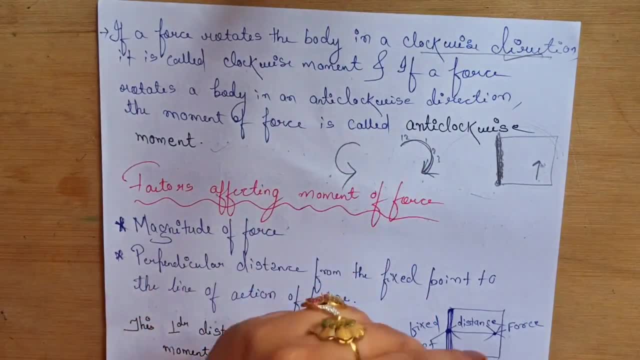 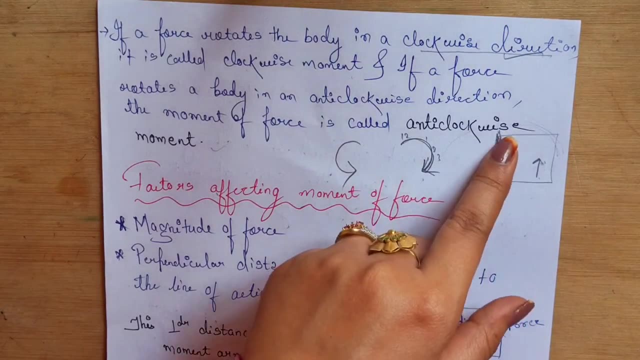 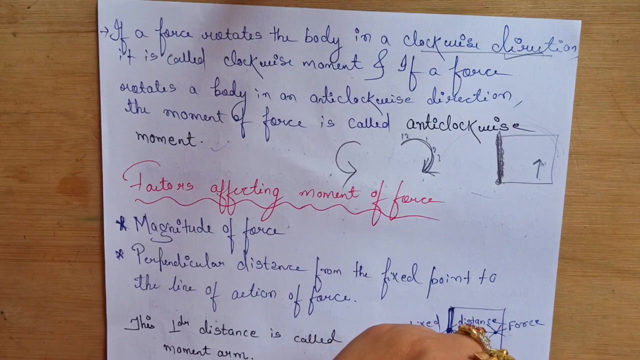 And you have to remember in this That the movement of force, In this The body, is not free. The body is fixed in one place. See, this body is fixed here. So if you are forced, The body will not rotate in a straight line or straight direction. It will rotate. 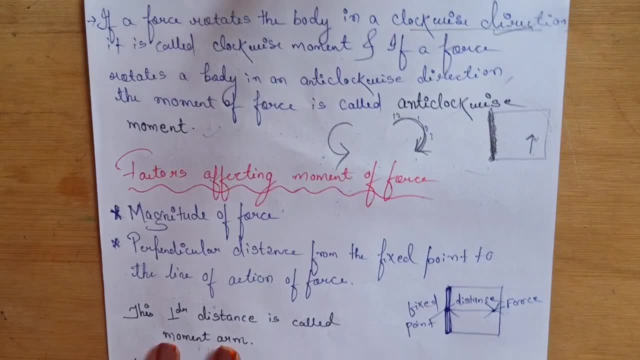 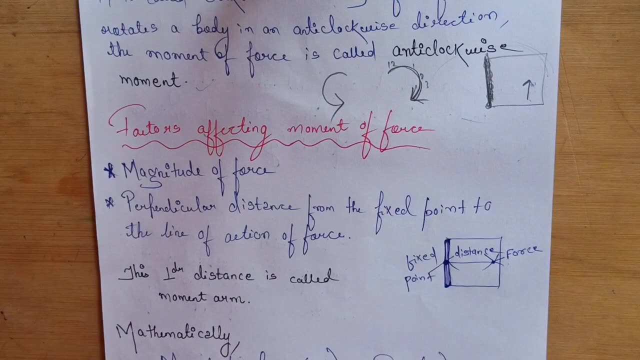 Means, The body will turn, The turning effect will be produced in that. Now, factors affecting movement of force. Now, what are the factors Because of which the movement of force Some changes can come, Or in which the movement of force depends? This is the meaning of speaking. So, this movement of force, 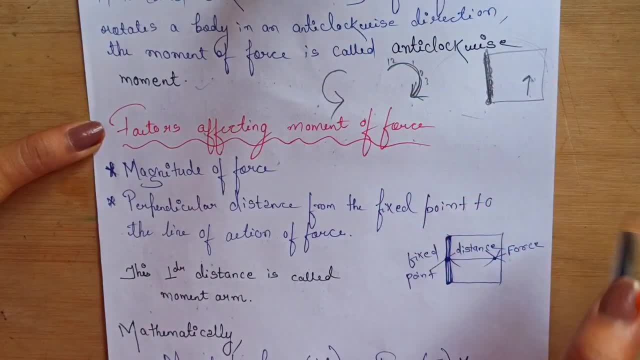 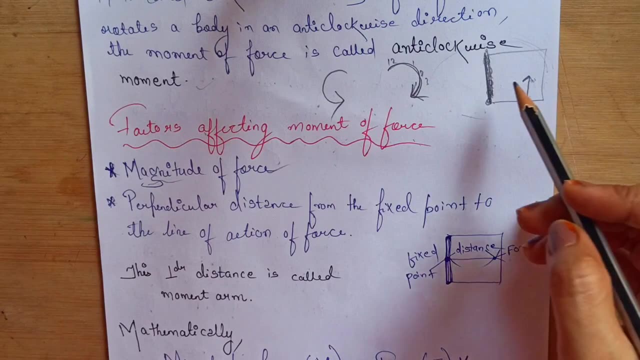 The turning effect that has been produced. That depends on two things. First, in the magnitude of force. Magnitude of force means How much force you are giving or how less. In that The more force you give, The more the turning effect will be, Yes or no. The more force you give in this door. 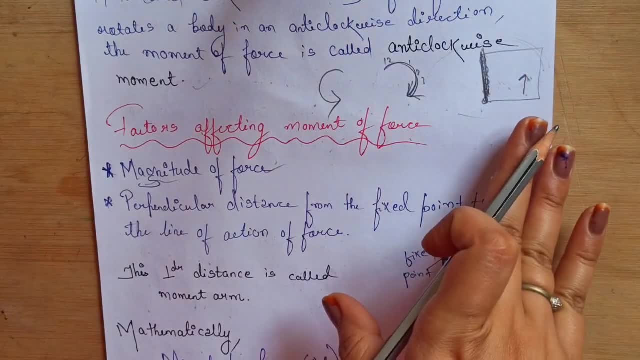 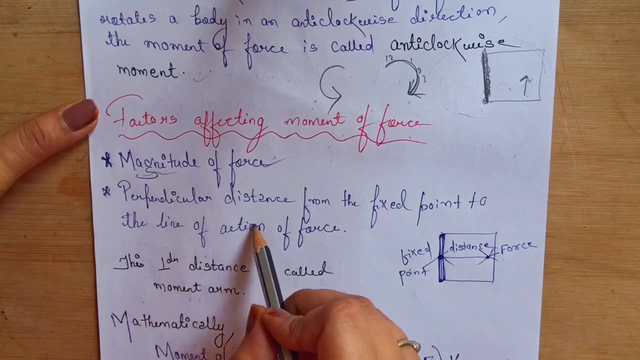 The more the door will turn, Yes or no. If you give a little force, Then it will be a little. If you give more, Then it will be more. This is the meaning of speaking. Then the second one depends on Perpendicular distance From the fixed point To the line of action of force. 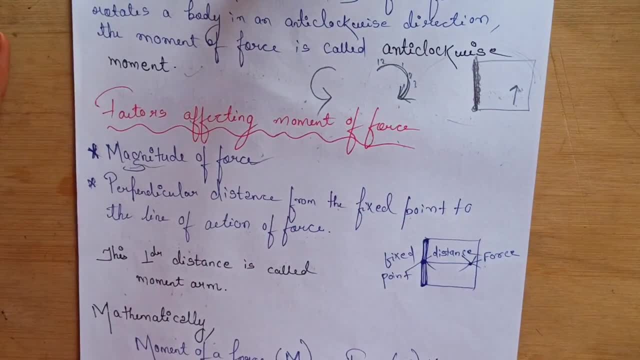 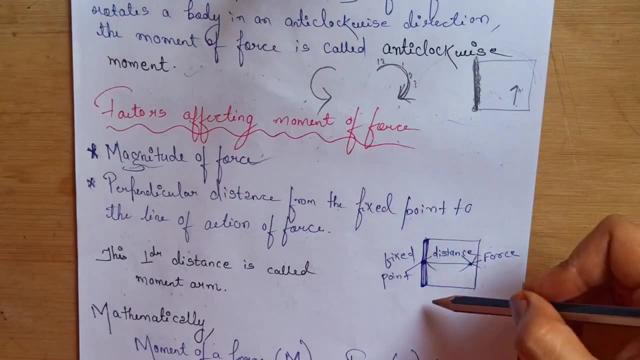 Now, this line is a little important And no one must have understood this. Now see, To understand this, You have to see this diagram Like: this: is the door. This is the fixed point in the door. This is the fixed point. So I write the fixed point like this: 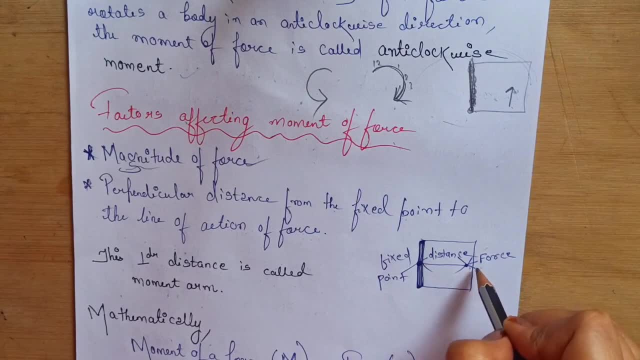 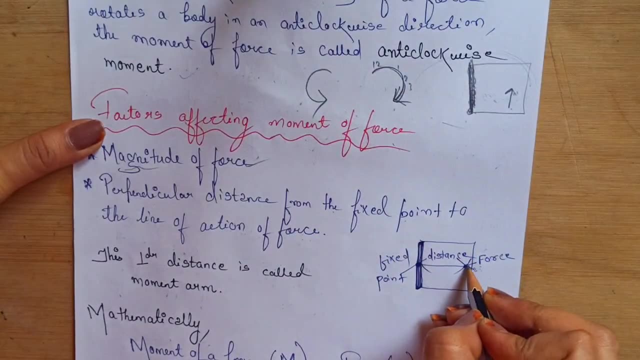 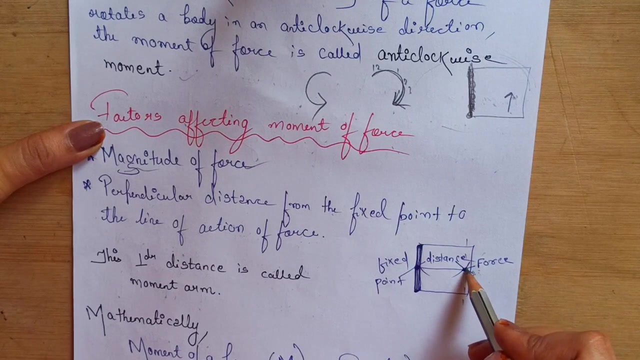 Now suppose you are putting force here, Where In this point, In this point you are applying force. If you are applying force here, Like you apply force in this point. So I am drawing a dotted line straight from here. So this line, Which is passing The point from which we are applying force, 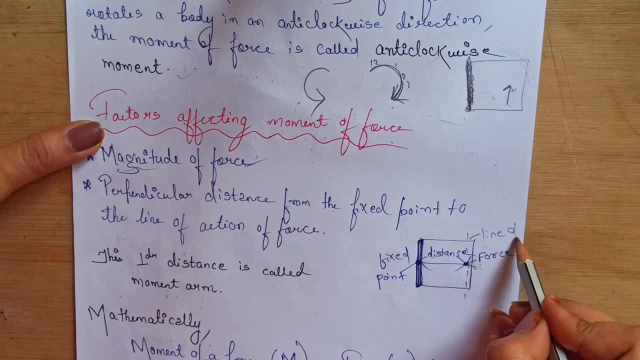 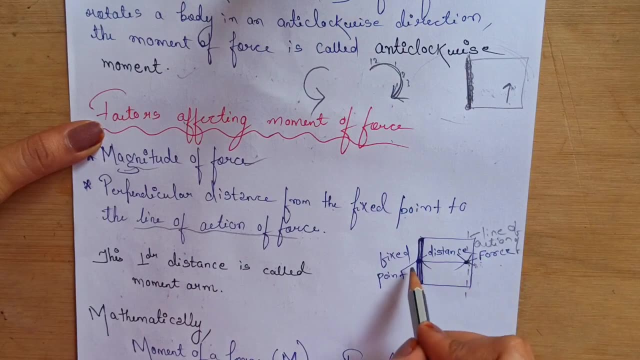 That line is called Line of action of force. Line of action of force Because the word is written here. That is why I mentioned that thing here. Ok, And this is the fixed point From where the object will be fixed. Now, This movement of force, What does it depend on? 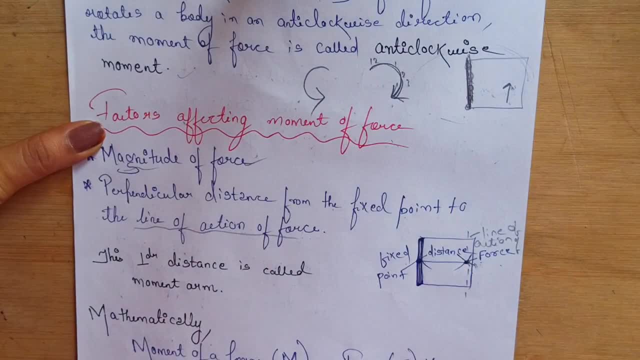 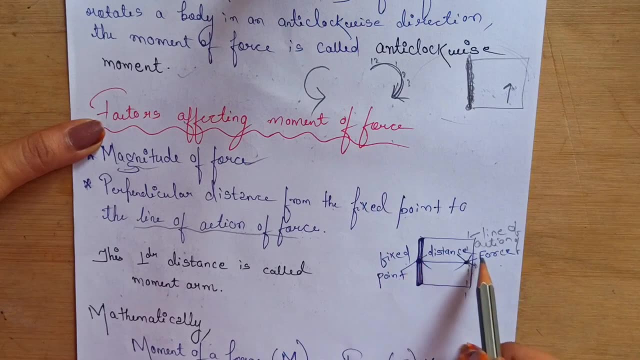 Perpendicular distance, That straight distance, Perpendicular, That number, degree is made. That is what we call Perpendicular distance. From where to where, Between whom, Fixed point And line of action of force If you are applying force here, And this is the fixed point, So this depends on the distance. 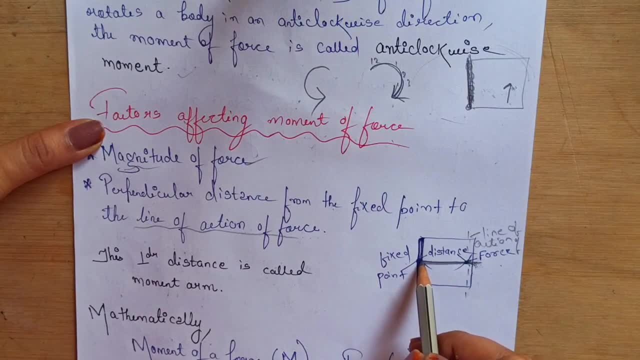 Your turning effect. Movement of force, This distance, Children, More, More, More, More Turning effect Will be produced. If Less distance Is the force from the fixed point, Less Less Turning effect Will be. For example, You go near the door of your house. Ok, Now children, You Who have this door. 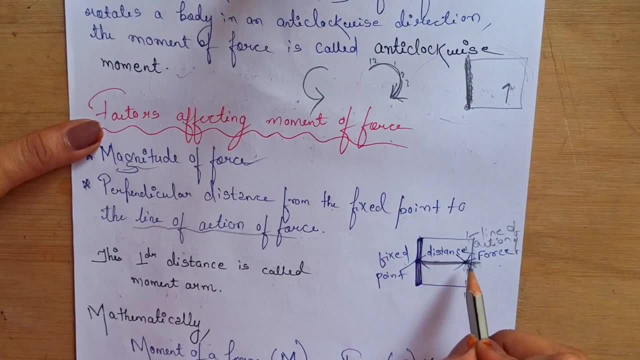 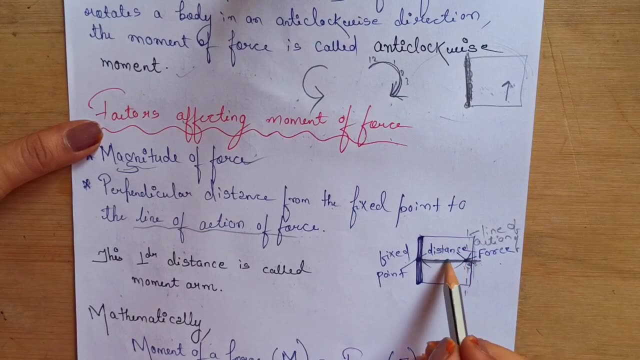 Knob is given here. So you If you force here, This is fixed point And here You are applying force. You, If you force, So easily The door will open. If you try to go near the fixed point and try to open or push the door, it will be difficult to open the door properly. the turning effect will be very less. 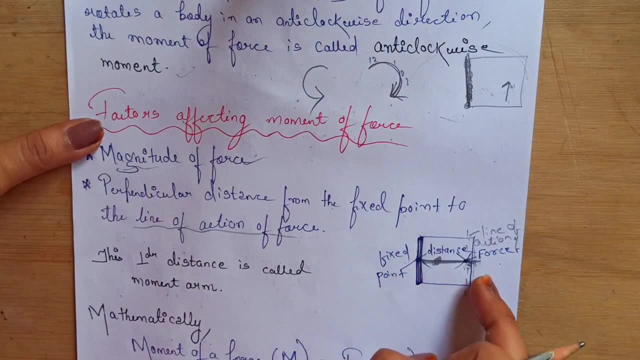 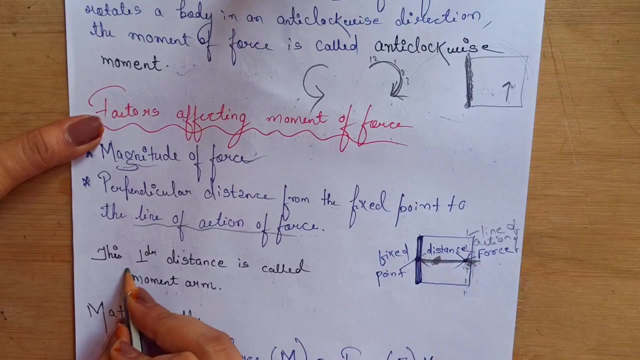 This means that the more the distance of the fixed point and the line of action of force, the more the turning effect and the moment of force will be seen. The less the distance, the less the turning effect will be seen. The perpendicular distance of the fixed point and the line of action of force is also given a name. it is called the movement arm. 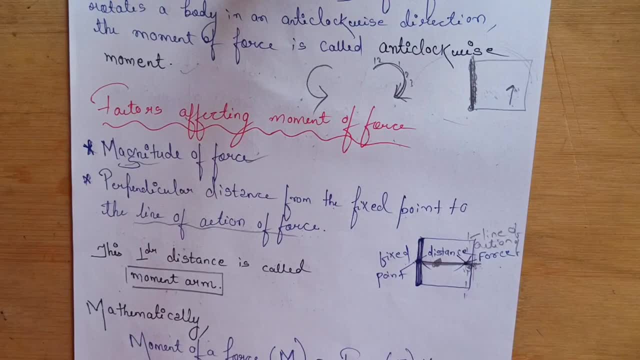 What is the movement arm? It is the distance, but the name given in it is the movement arm, so you have to remember this name. What is the movement arm? It is the distance between the fixed point and the line of action of force. 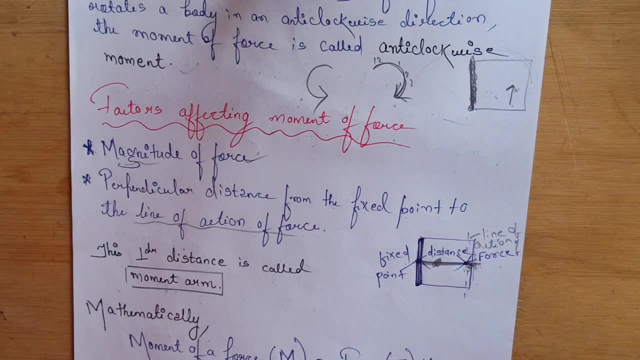 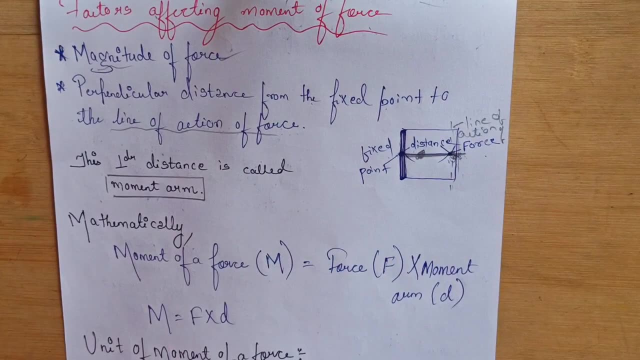 We can call this movement arm by another name If we want to show mathematically or if I say that if I make a formula of the moment of force, then the moment of force is normally shown in this way. The moment of force is normally shown in this way. 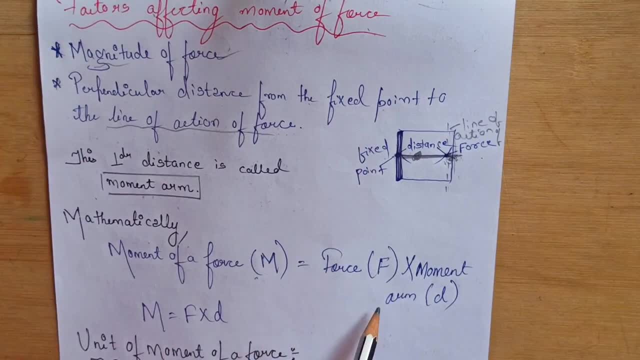 What is the formula of the moment of force? It depends on two things. just read it. The moment of force is the magnitude of force and the perpendicular distance, which is called the moment arm. What is the formula of the moment of force? 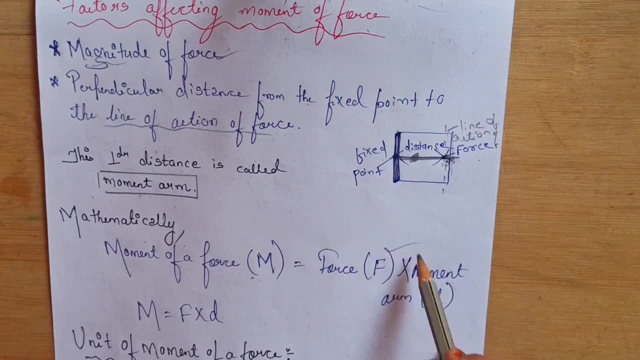 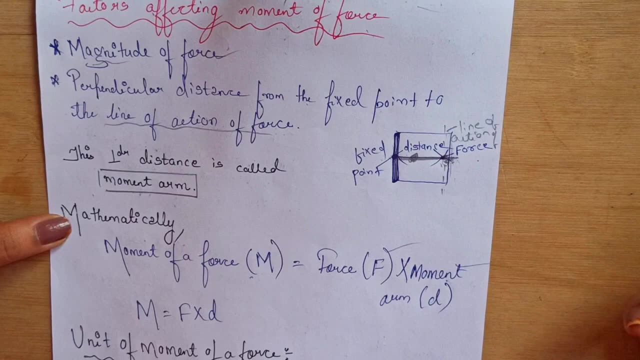 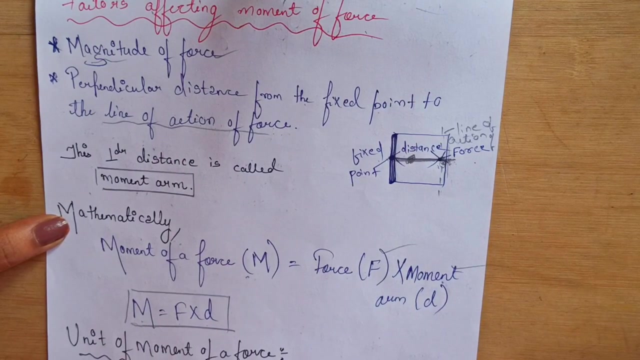 It is the force into the moment arm or the force into the perpendicular distance between the fixed point and the line of action of force. We can write it as: m is equal to f into d. This is also the same formula. m is equal to f into d, where m is the moment of force. 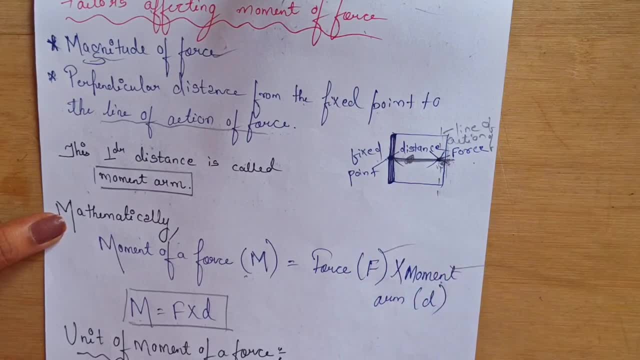 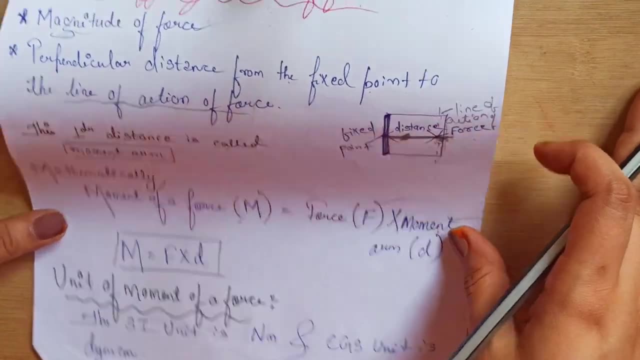 f is applied force and d is the moment of force. If we try to find out the SI unit of this, then we can find out the SI unit of this. We can also find out the CGS unit of this. SI and CGS are very simple. 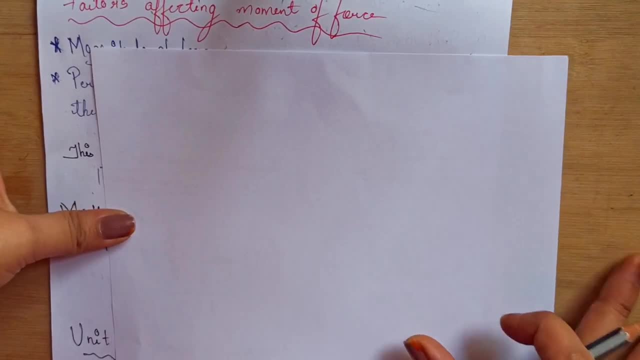 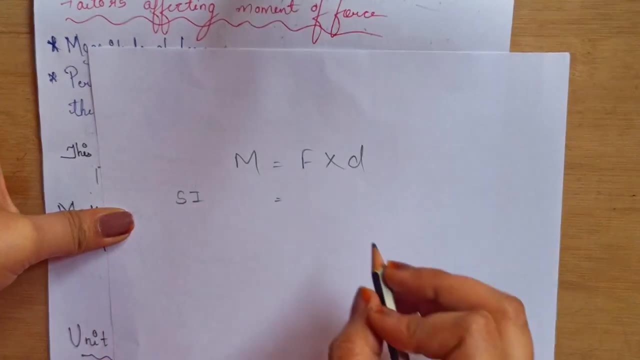 First let's write the formula. You know how we can find out the unit of this without making a mess. m is equal to f into d. If I talk about the SI unit, then first write the formula. What is the SI unit of force? 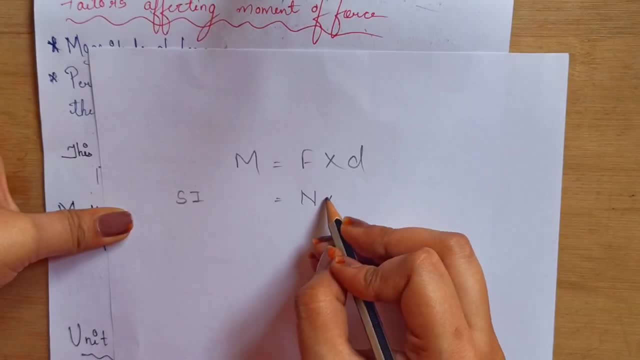 Because there is force in the formula. Let's write Newton. Let's write Newton into What is this Distance? The moment arm is called distance. What is the unit of distance? SI unit is meter, So its unit is Newton meter. 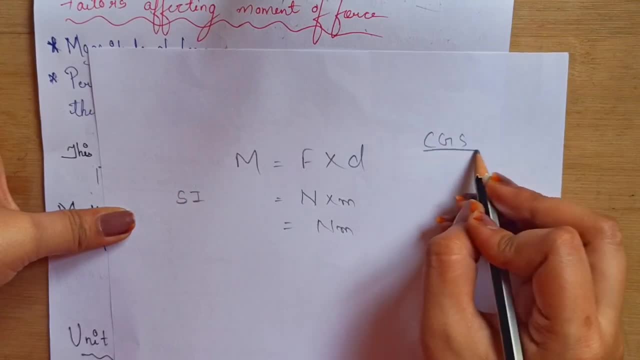 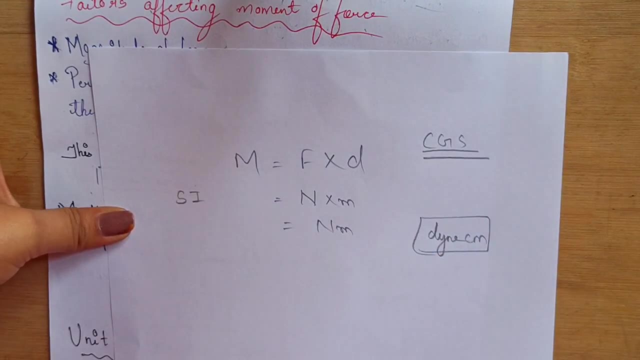 This is its SI unit, And if I talk about the CGS, then just change the CGS Dine in place of Newton and centimeter in place of meter. So this is its CGS unit. It is very simple. With the formula you can make any unit of anything. 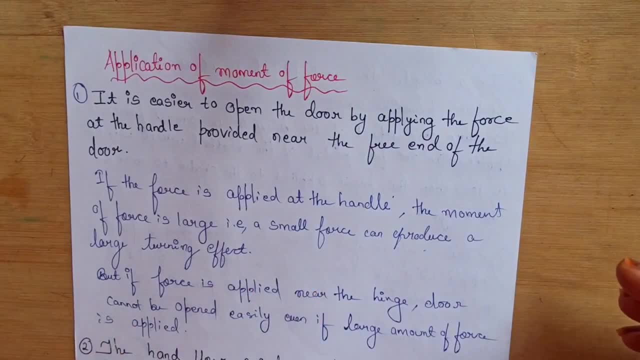 It is very simple. Okay. Next is application of moment of force. Now, this moment of force. This is applied in our day to day life. Listen carefully, children. Okay, Now, as I said earlier, same thing: It is easier to open the door by applying the force at the handle. 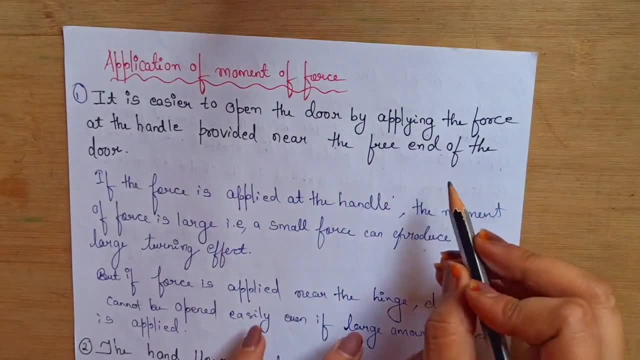 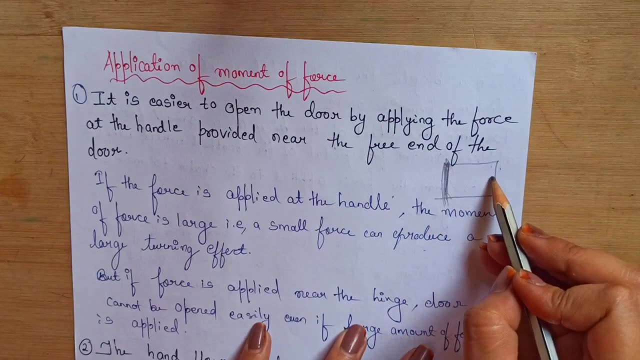 Which is provided. near the free end of the door There is a door. Your door is fixed from here And this is the free end If you want to open the door. So if you are applying force near the free end, then the door will open or close very easily. 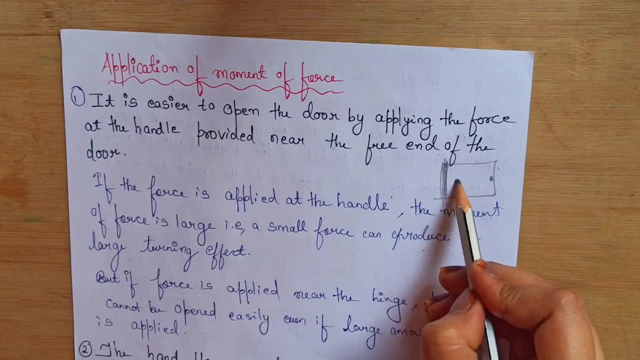 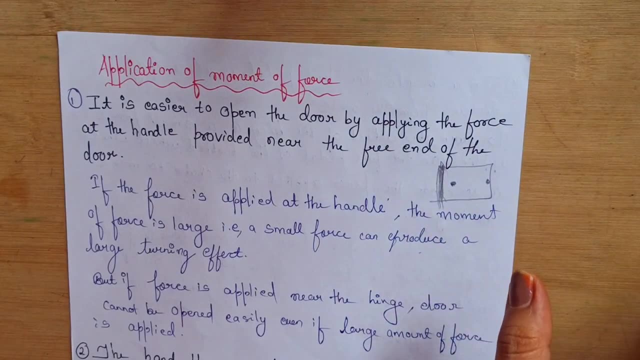 But if you are applying force near the fixed point, If you are trying to open or close the door, If you are applying force near the fixed point, Then it is difficult. Difficult means it will take a lot of strength. Speaking means it will take a lot of strength. 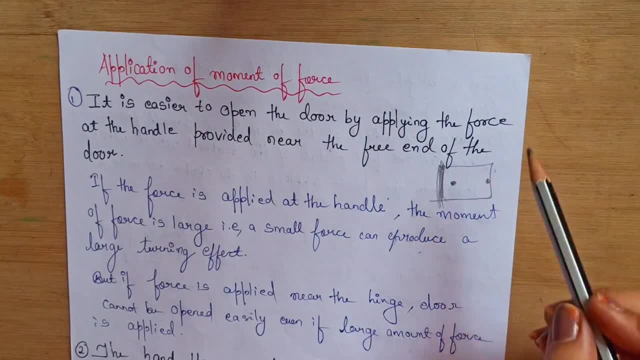 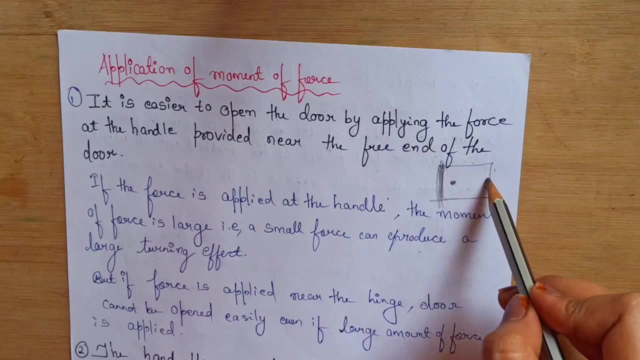 Right Now. listen carefully. what is its explanation Here? it is saying that if we apply force in the handle, Handle is here. If we apply force in the handle, Then here the moment of force is large. The moment of force is large means the turning effect will be very high. 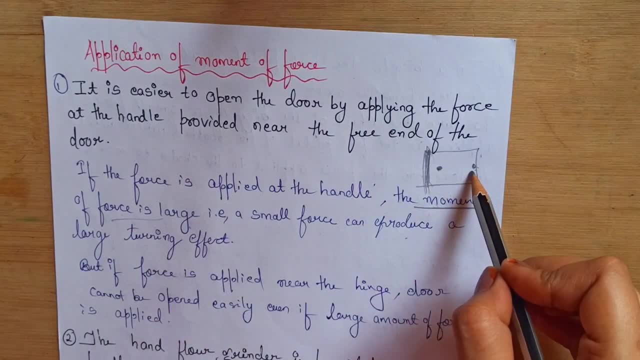 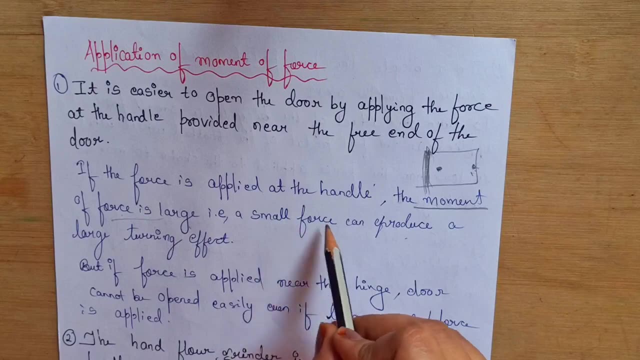 The moment of force is large means the turning effect will be very high. If we apply force here, then the gate will open easily. It will turn well, And here small force can produce a large turning effect. That is what it means to say. 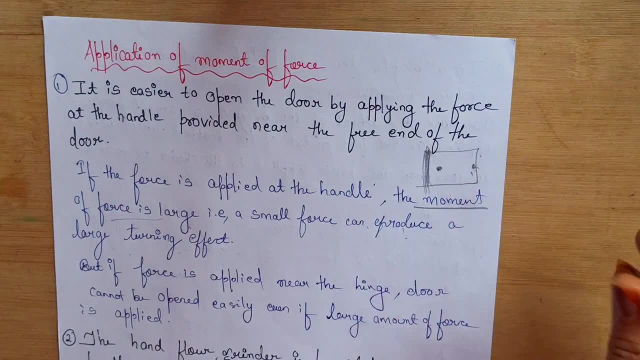 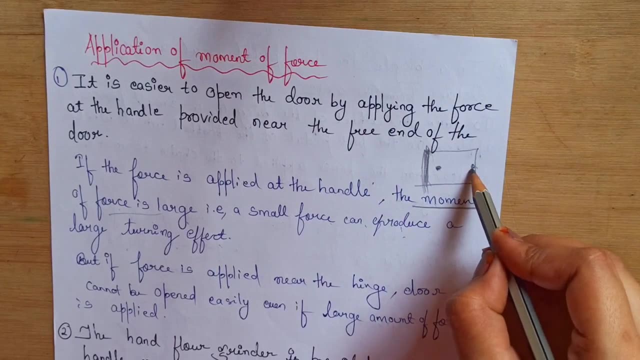 That if we apply force here, Then small force, You can produce a large turning effect by applying a little force. Yes, you don't have to apply a little force. You apply force here And your gate will open easily. Speaking means it is. 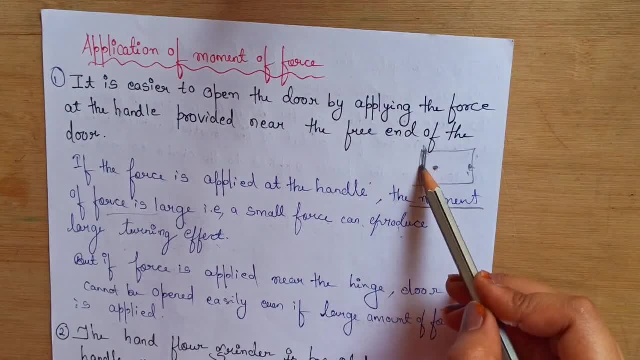 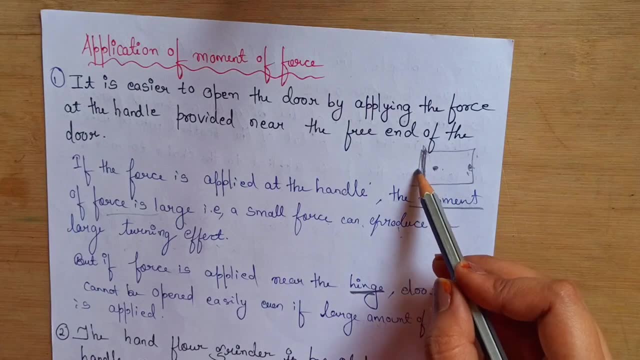 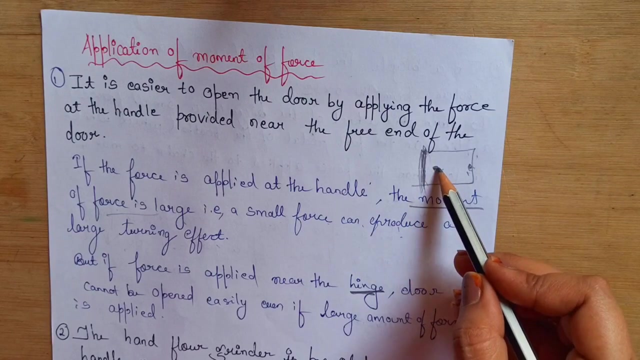 But Now, for example, if you are near the hinge, These are called hinges. The word written here is hinge. It is called this If you are applying force near the hinge Here, So in this case Our door will not open easily. 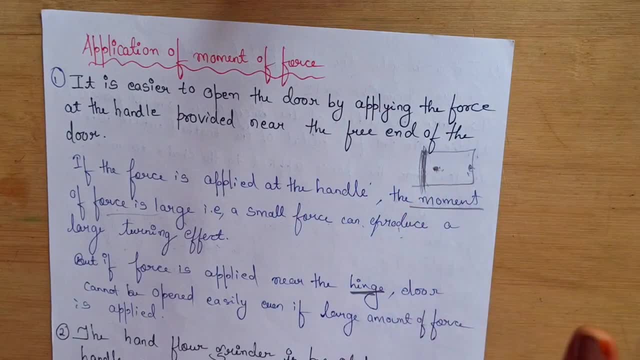 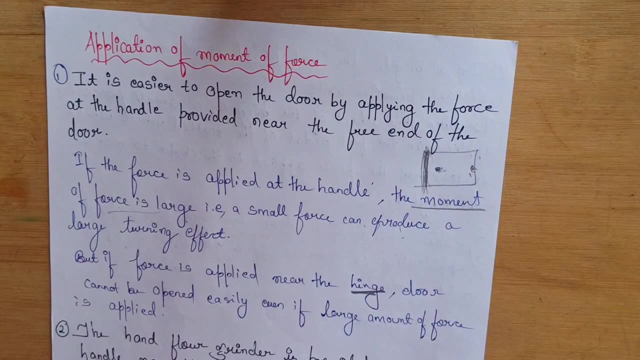 It will not open easily, No matter how much force you apply, But easily turning effect. Not much turning effect will be produced, But in this case, in a little force, The last turning effect, This moment of force, You get to see more. 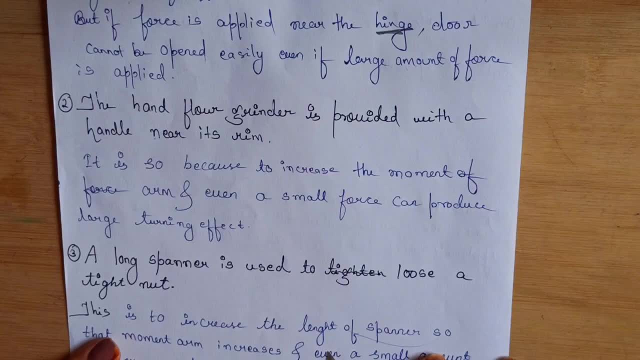 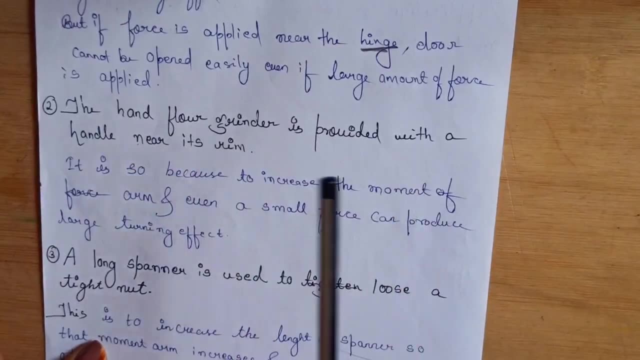 But this is the only explanation in it. There is nothing else. Very simple. Now the second application of this is given. The hand floor Grinder is provided with a handle near its rim. We grind the flour, Not the flour, Sorry. 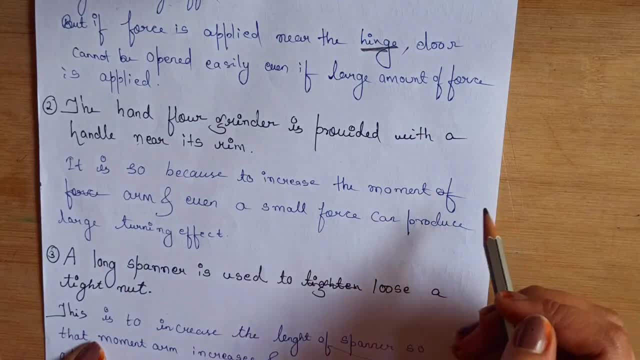 We grind the wheat With which the flour is made. That is the grinder, That is the mill. Okay, Gandhiji used to run The mill for grinding wheat. The mill, That mill is there. Suppose it is a mill. 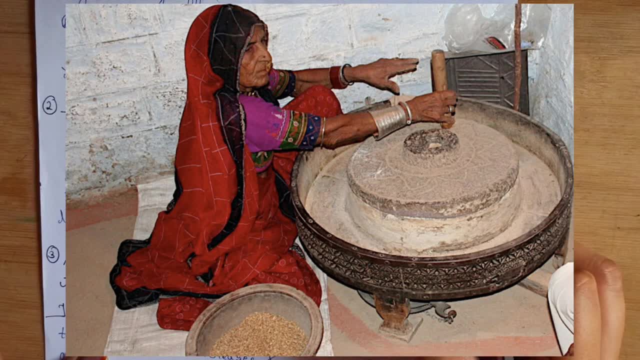 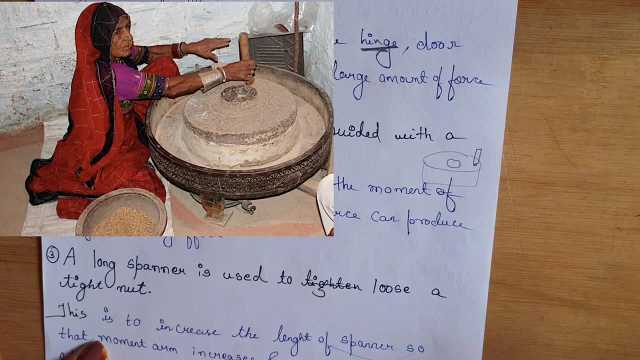 He is saying The handle of it It is given here. Rim means corner side, Here, Here And here in the middle. It is like a hole. There we put the flour, Not the flour, There we put the wheat. 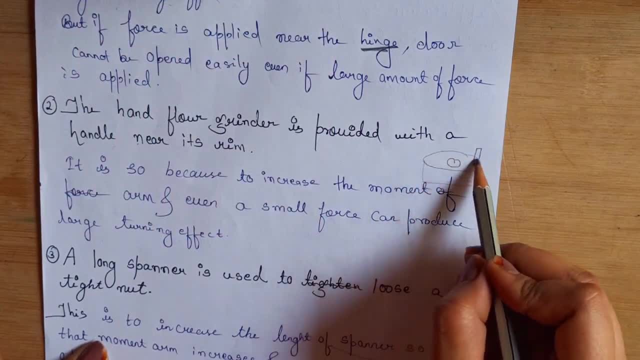 Okay, Here we put the wheat And hold it from here, Rotate it like this So it converts into flour. Now here it is saying: Why does it give its handle on the side? It is very important Children Give it on the side. 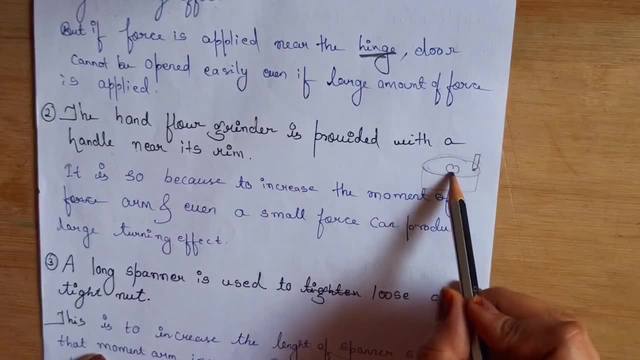 Okay, Its handle. Now, this is a fixed point. What happened, Fixed point happened And from here we are applying force, Because we will hold it from here and rotate it. So here we will apply force And this is our fixed point. 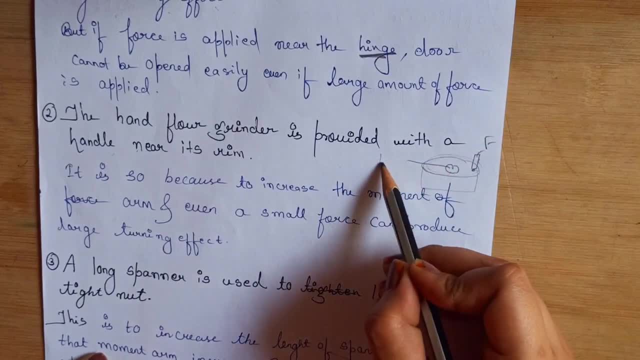 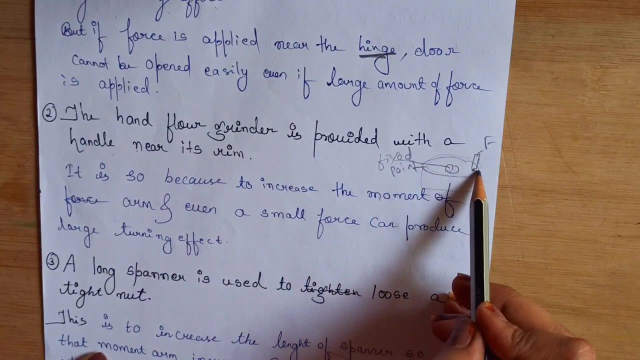 What happened? This is a fixed point Now From here. This is a fixed point Here. we will apply force. So between the two, We will apply force Now. This is a fixed point. Here we will apply force. So between the two. 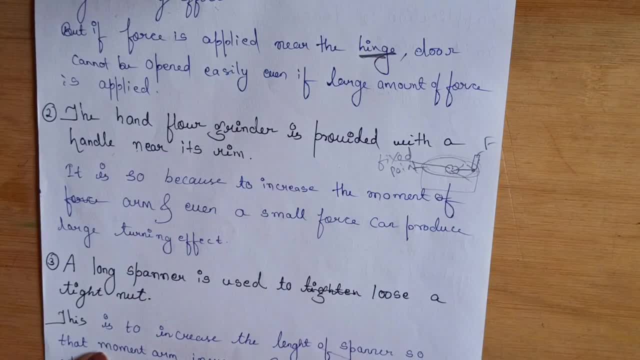 There is some distance. In my diagram There is a small distance, But normally there is a distance. Okay, When this distance is kept well, And this step is applied from the side only, So that If we apply a little force. 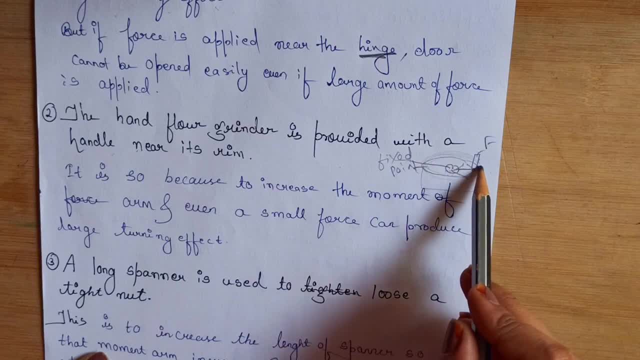 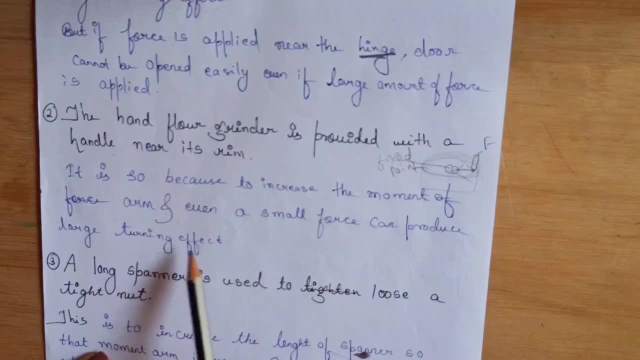 Then more turning effect will be produced, Or there will be. It is so because to increase the movement of arm And even a small force can produce large turning effect. Why is it given If the distance between this and this will be more? 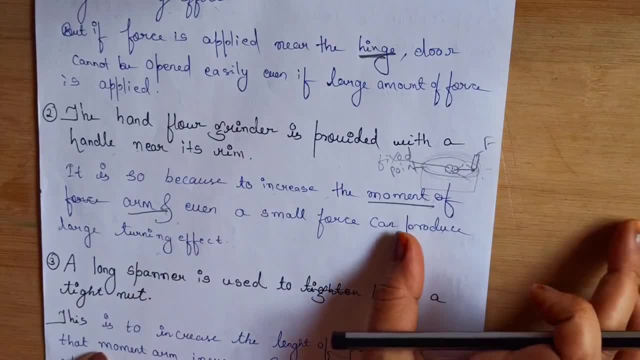 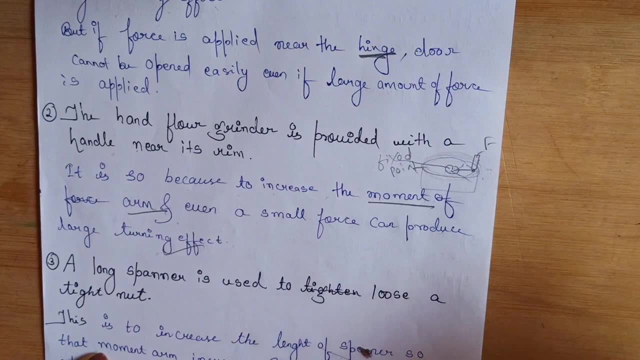 Then the movement arm is more. Distance is more- Okay, Yes, which means it increases the movement time, due to which, if you force it a little, then the last turning effect will be produced, but if the distance of these two is very less. if it was near here, then we would have to apply a lot of force. 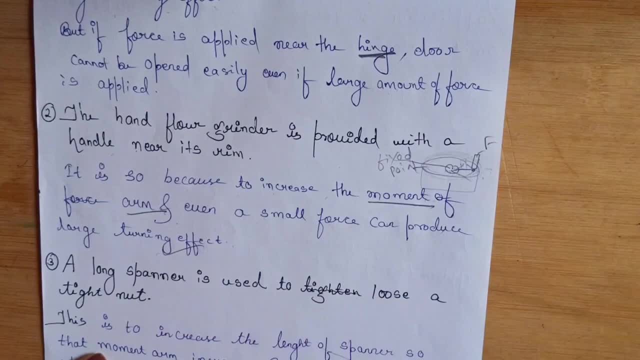 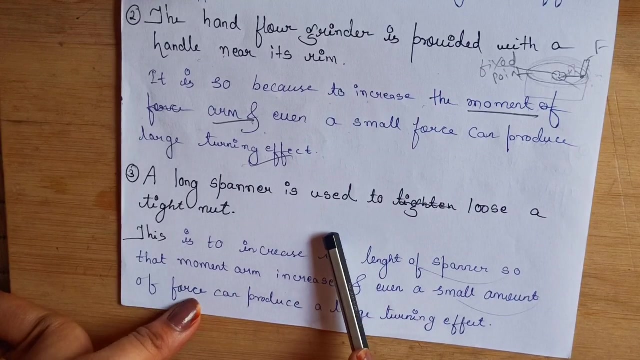 little force does not work. yes, we have to apply force in this too, but here the distance is more, so the last turning effect can be produced by small force. see, the science is applied now. third application: a long spanner is used to loose a tight nut. a nut is very tight. 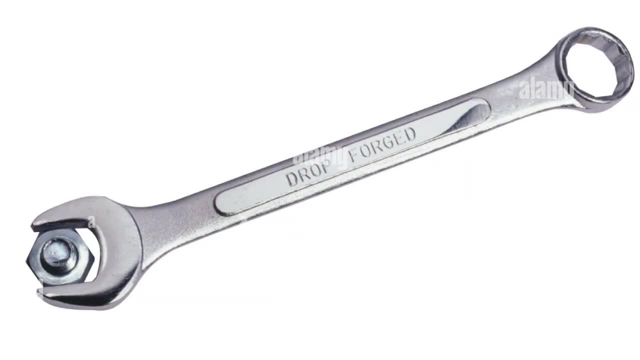 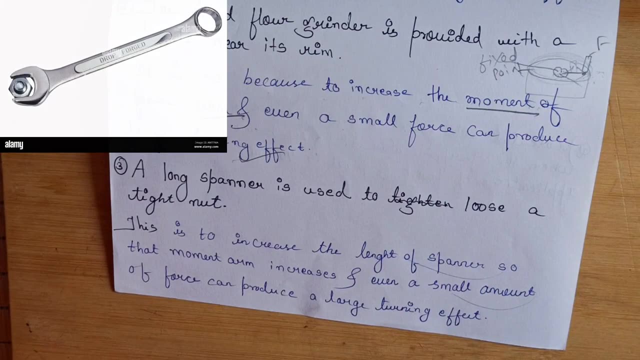 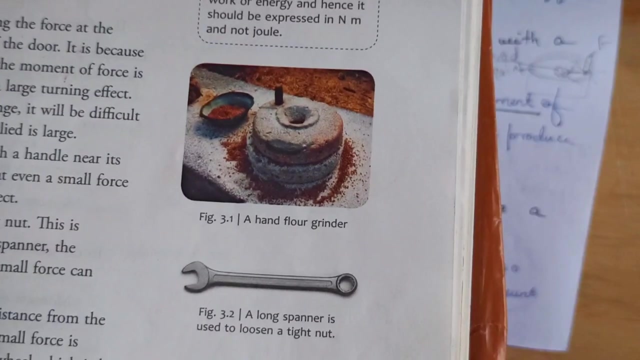 see the photo on the side. this long spanner is used so that we can loose a tight nut. so here we are talking about a spanner. so why is the spanner so long? I will show you in the photo here. it means that this is how long it gives. 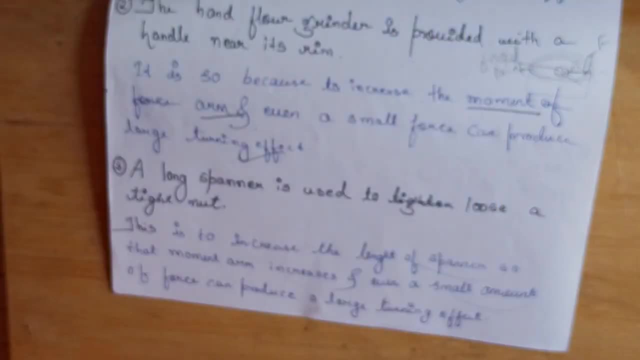 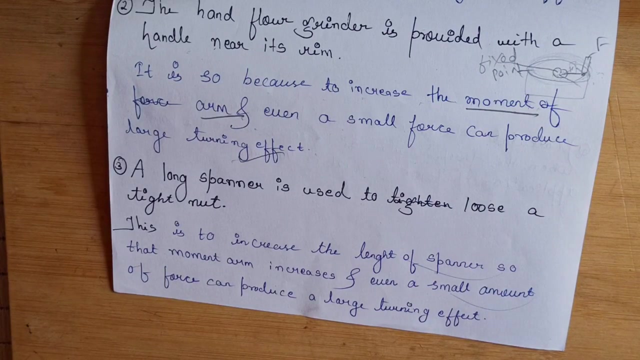 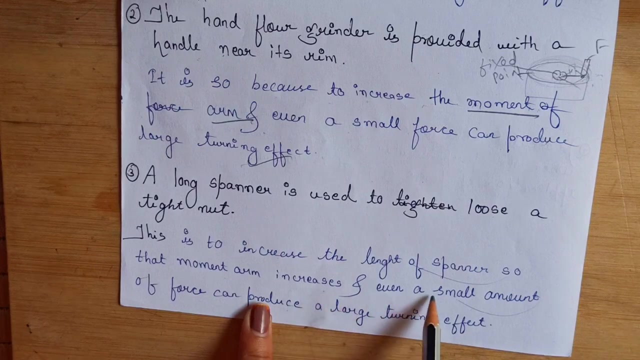 so long. spanner is used. here also the same turning effect and movement time is being talked about here. also the same expression is there. why is it done? to increase the length of spanner, so that movement time increases and even a small amount of force can produce large turning effect. 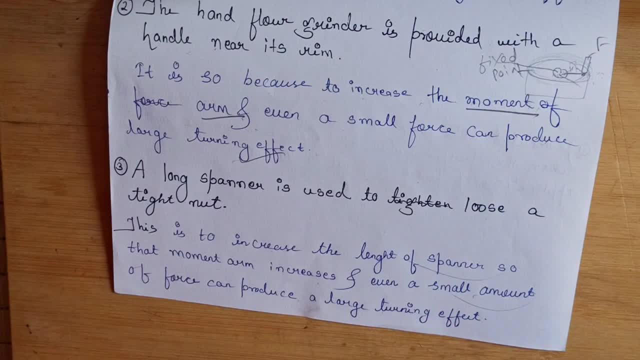 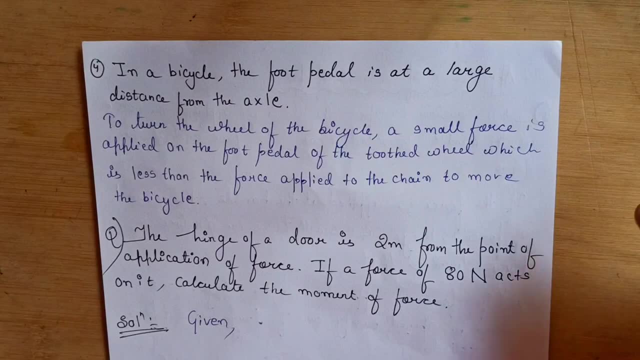 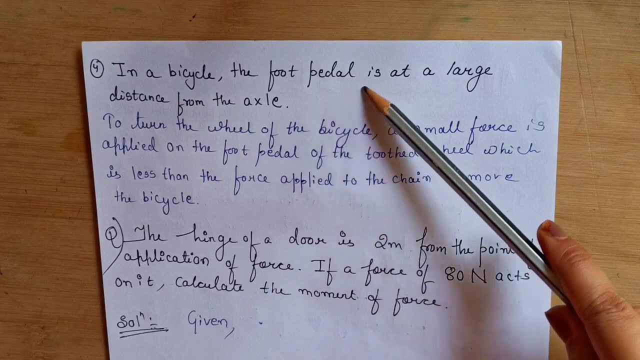 it will be long. that means movement time will increase. so we are producing more turning effect with little force. otherwise there will be no problem now. the fourth application is related to bicycle. it is related to cycle. in cycle, the foot pedal is at a large distance from the axle. 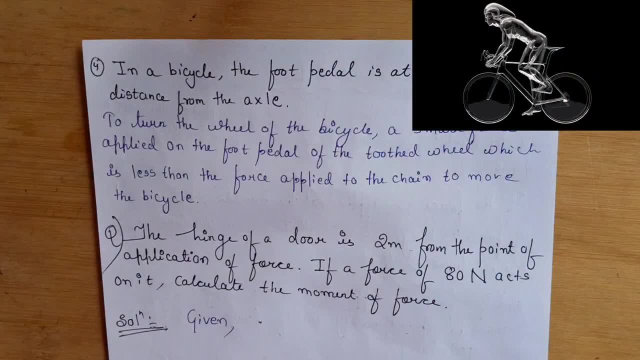 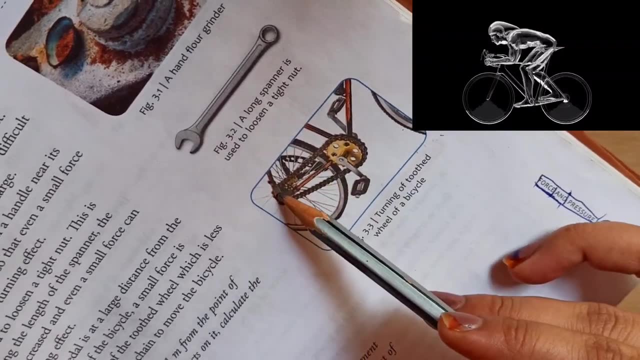 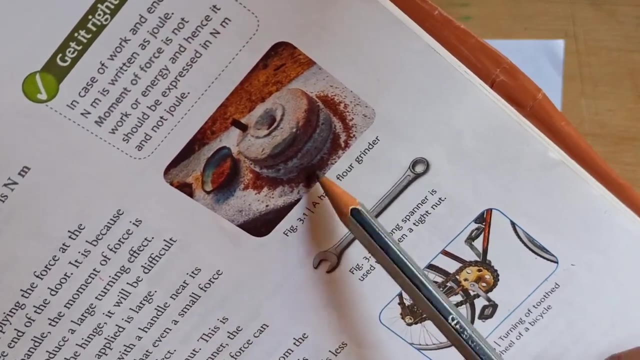 if I show you the diagram. so this foot pedal- see, this foot pedal- is at a large distance from the axle. this is also given due to a reason. earlier we have read about grinder- hand floor grinder- is that distance is more here? leave it first, let's see this. 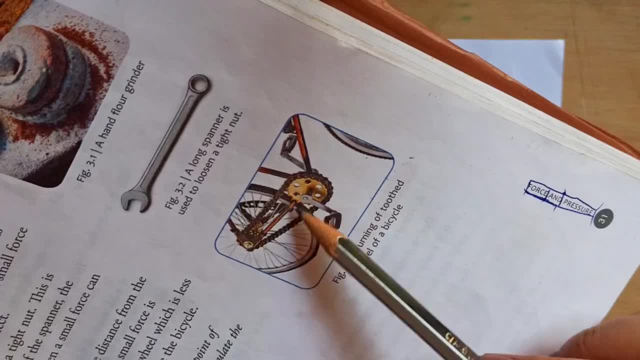 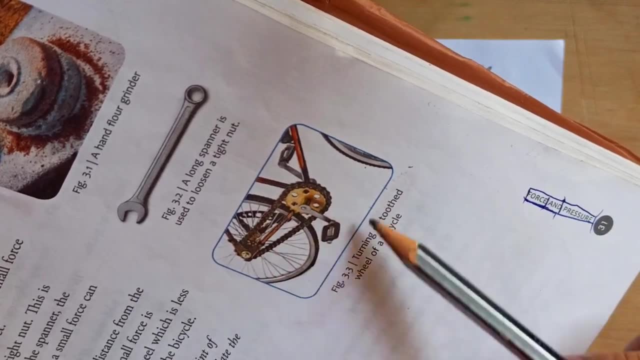 that topic is over. so here the foot pedal has a good distance from the axle. what will be the reason? same movement time increases, so more turning effect will be produced than small force. but if these two are very close, if this pedal and this are very close, 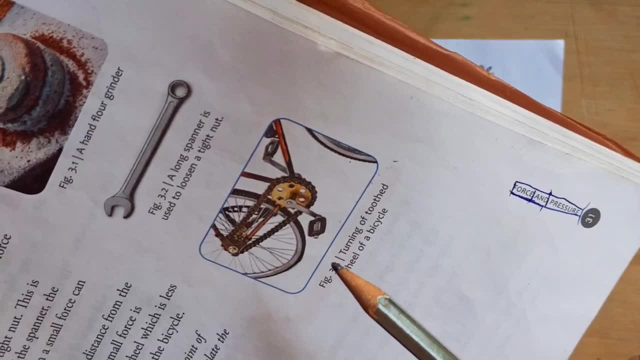 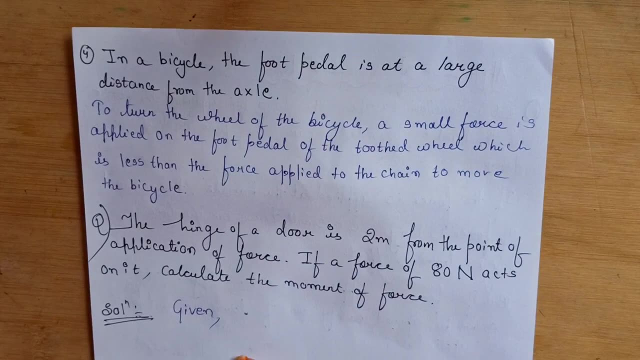 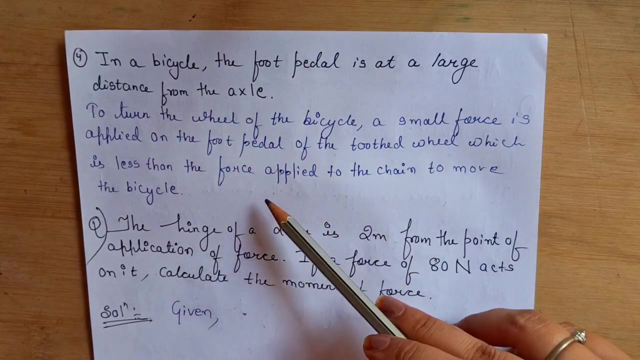 then we have to apply a lot of force and despite that, too much turning effect is not produced. ok, so its reason is here. now let's discuss. to turn the wheel of a cycle, a small force is applied on the foot pedal of the toothed wheel, which is less than the force applied to the chain to move the bicycle. 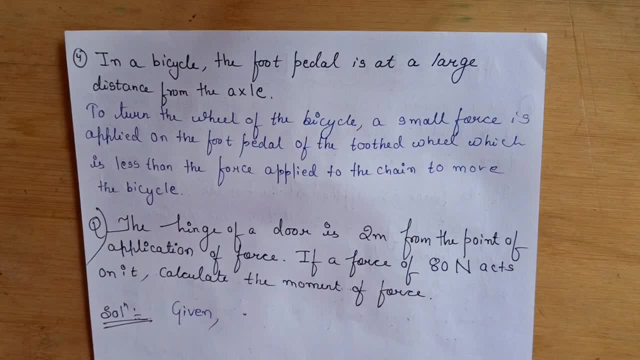 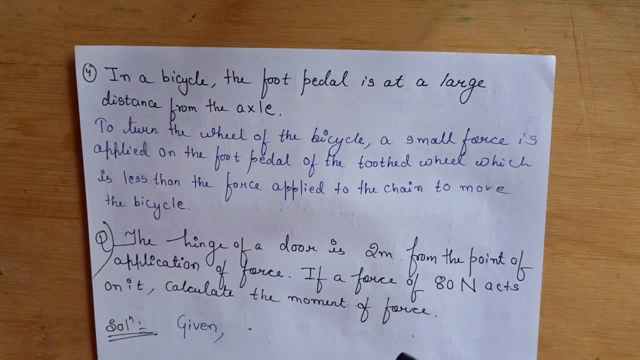 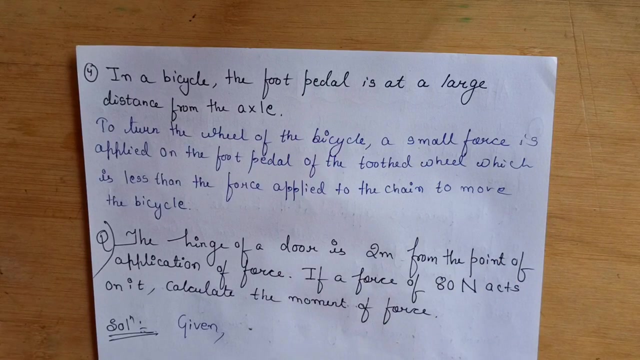 what I have told you. same thing is given here. now we will see its numericals. ok, we will see its numericals, but before that let me tell you, in this case, as we explained earlier, that we increase the movement time, so small force can produce large turning effect. 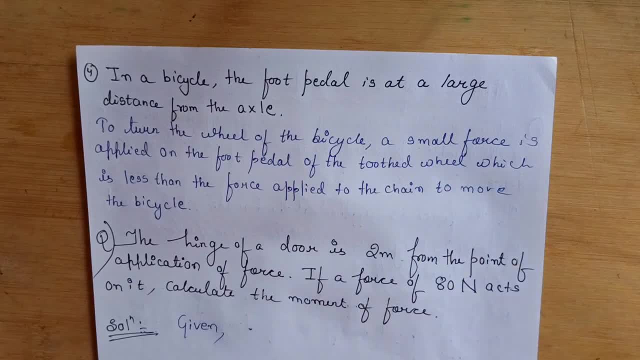 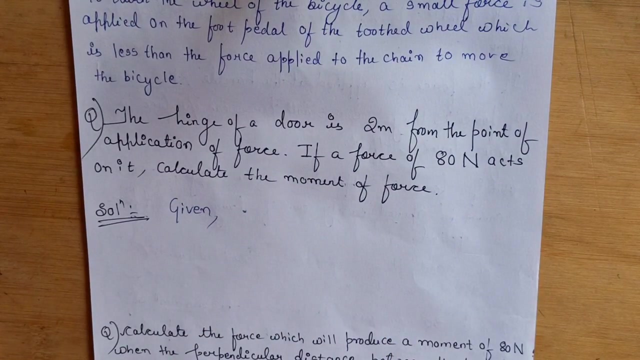 you can write that too. if someone is feeling this stuff, then you can write that too, because the application of movement of force in this maximum place means in maximum place. the explanation of the reason goes the same, so don't take so much tension. now let's see some numericals. 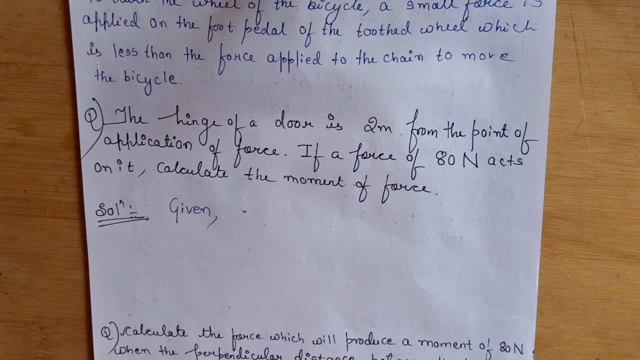 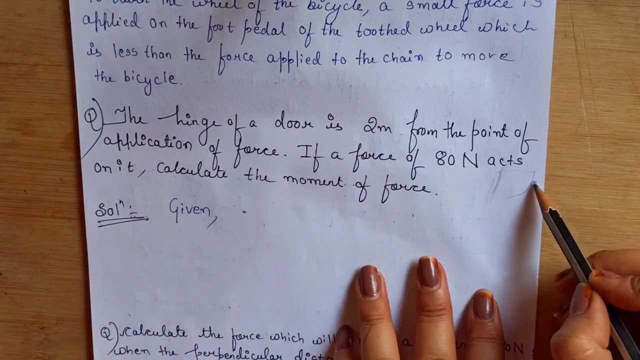 the hinge of a door is 2 meter from the point of application of force means the question is the hinge of the door. the hinge of the door is the application of force, where force is applied. so its distance is 2 meter. so what we have given is: 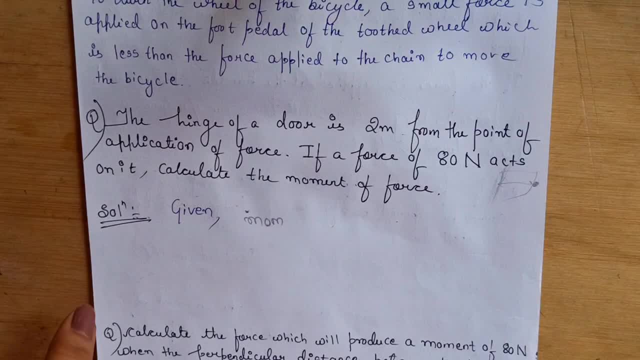 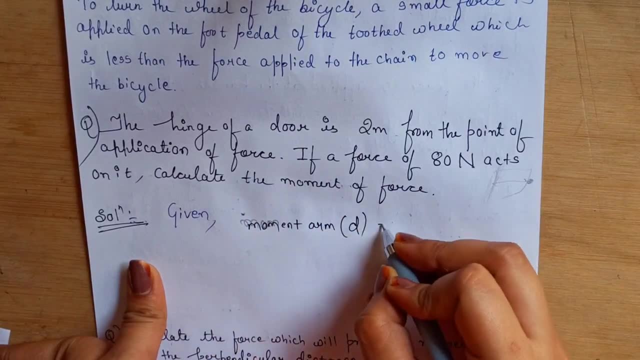 movement. wait, let me use the pen. so what we have given is: we have given movement arm, we have given distance, so we call it movement arm, we can call it, we can write it as d how much we have given 2 meter. ok, we have given this. 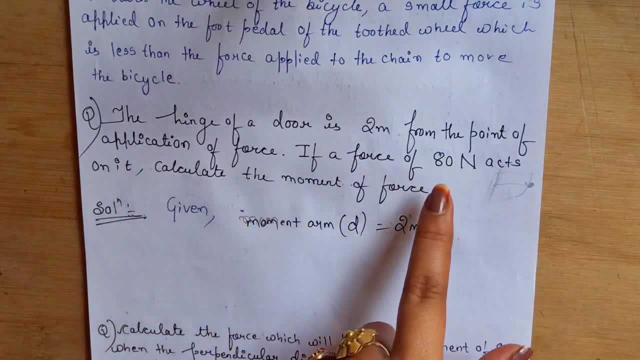 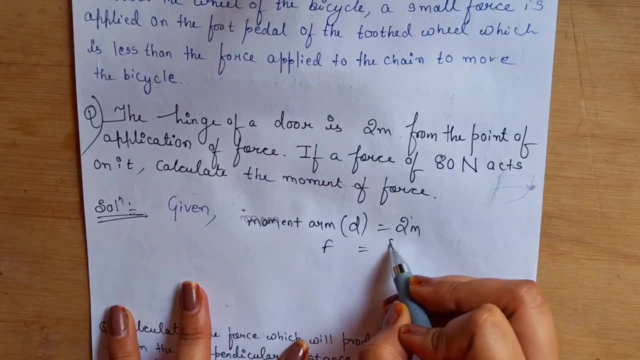 if a force of 80 newton acts on it, if 80 newton force is working in it, 80 newton force- so we have given force F is equal to 80 newton. it is saying: take out moment of force. so I can write moment of force simply as M. 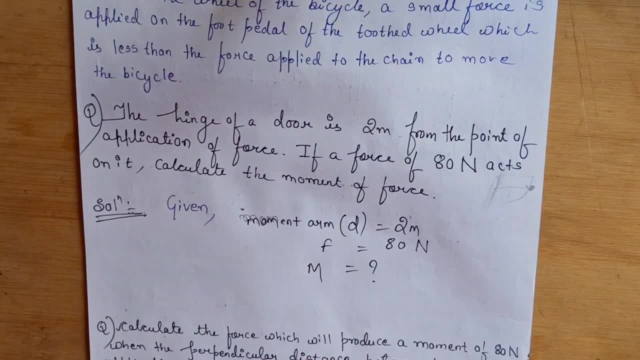 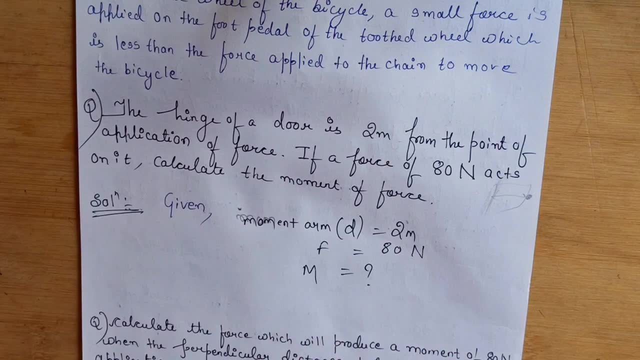 now, first of all, whenever you do numericals, read the question, understand what you have given, mention it. so here we have given moment arm, we have given force, we have mentioned what we have asked, we have put question mark in it. now the next step you have to do: 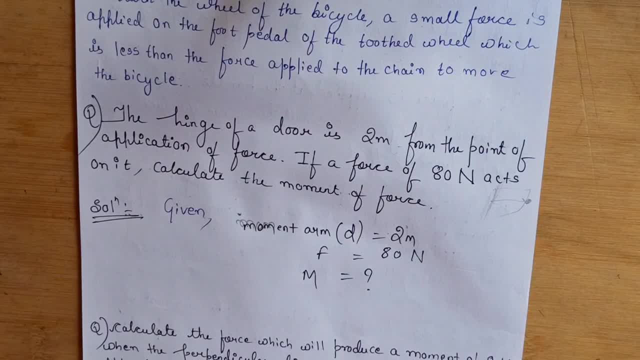 is to see that their unit is only one or not, like in SI unit. so both three should be in SI unit. if it is in CGS, then both are in CGS. so this is meter, this is newton. both are SI unit only there is no need to take any tension on it. 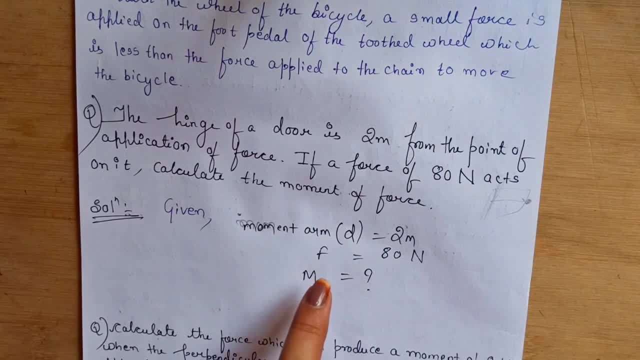 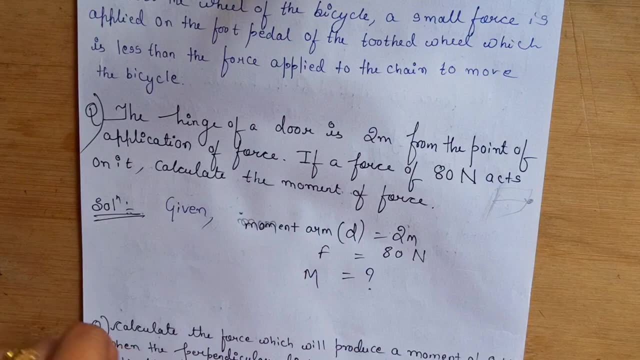 now see this formula in which moment arm also comes, force also comes and distance also comes, moment arm also, like moment of force also comes, force also comes and moment arm also comes. so we have read the formula. what is the formula? one minute. let me set it ok. 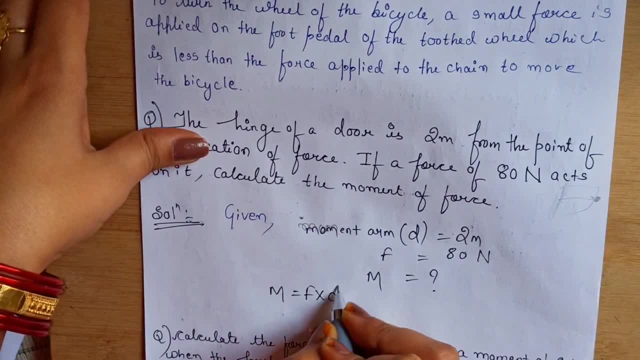 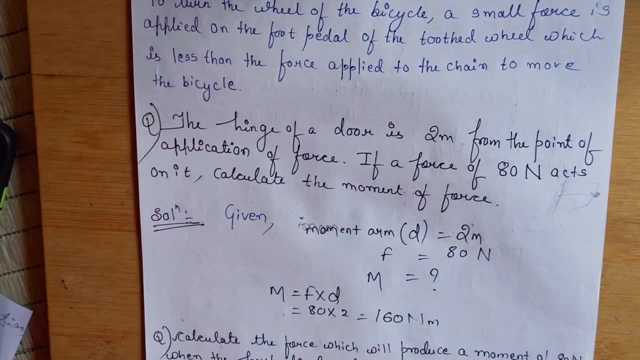 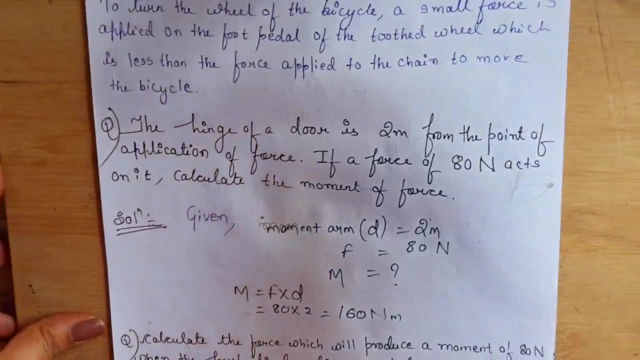 so what is the formula? M is equal to F into D. just write the formula, put the value and the answer will be 160 newton meter. very simple, 160 newton meter. so this is your first numerical done. similarly, let us see the second number: calculate the force. 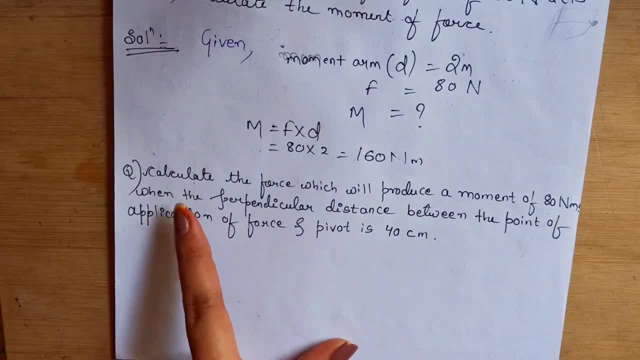 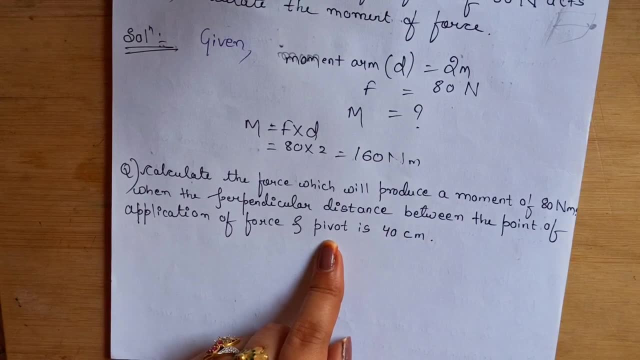 which will produce a moment of 80 newton meter when the perpendicular distance between the point of application of force and pi watt is 40 cm. this word, pi watt, is a fixed point. now, what is given in the question? it is asking to calculate force, calculate means. 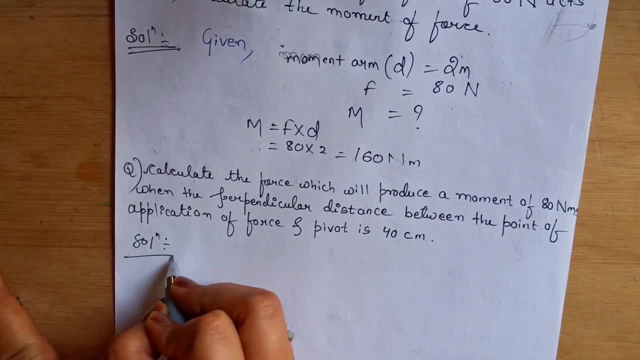 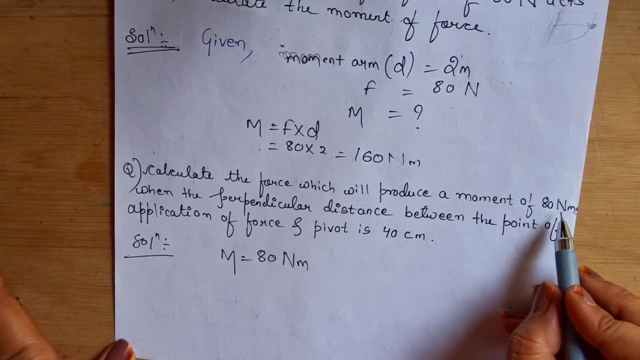 find. so it is asking us to calculate force. ok, we will do. moment of force is given. M is given 80 newton meter, and if you don't understand that this moment arm is given, then see its unit. it is given newton meter, so whose unit is it? 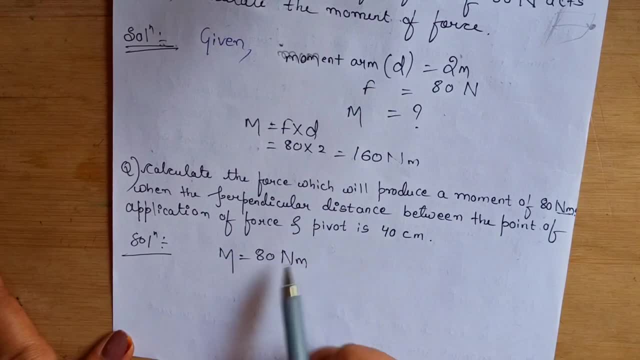 moment of force, perpendicular distance between application of force and pi. watt means this moment arm is given 40 cm. it is asking us to calculate force. now, in the next step, what we have to see is its units. now see units. it is in newton meter. it is 1 cm. 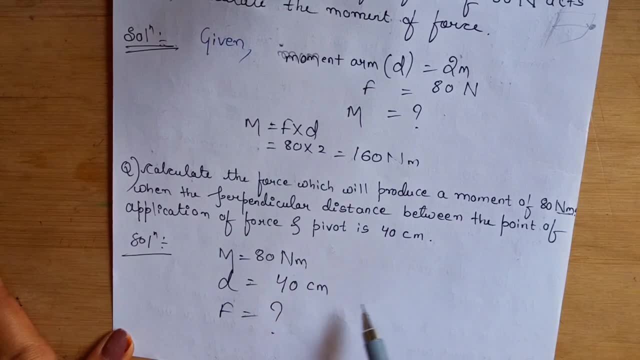 now here, if you are studying newton meter, it is same and cm is cgs, so we have to do both in the same unit. so how will we do? let's do one thing. let's do one thing. this cm is given in meter, so cm is given. 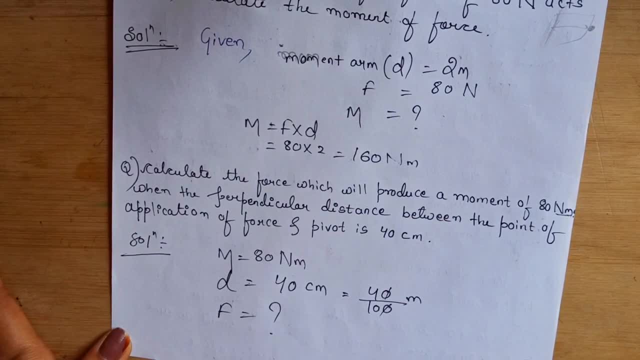 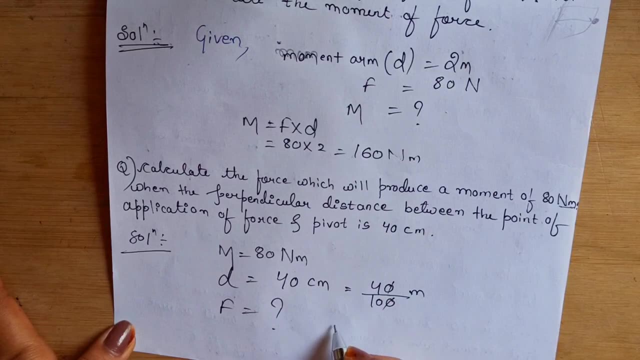 in meter divided by what? 100, so 4 by 10. if you want, you can solve it further, but I am leaving it this much. right now we have to calculate force, so first of all write: the formula: M is equal to D into F or F into D. 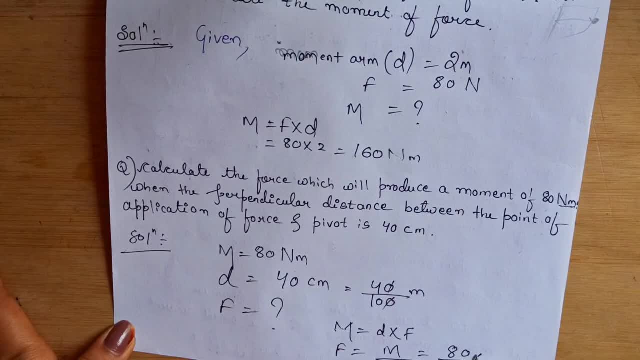 if we have to separate F, then M by D, M is given 80 and D is given 4 by 10, so that by 10 will go up, and this is force. so what is the unit of force? I can't see. I am doing it. 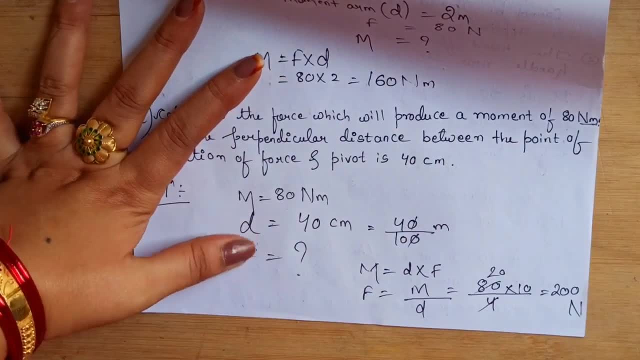 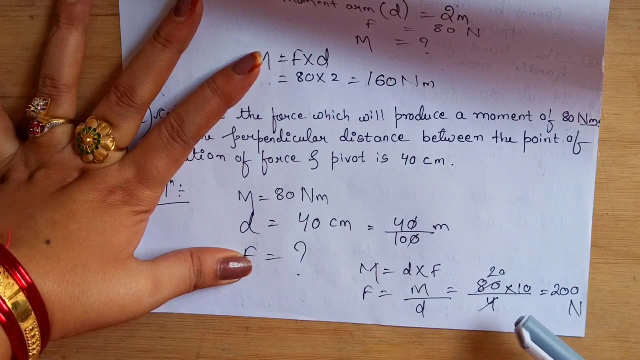 for a long time. no problem, I will show you ok here I have written the formula. force is equal to M by D. put the value of M, D was 4 by 10, so 4 is down and 10 is up. you must know this if we solve. 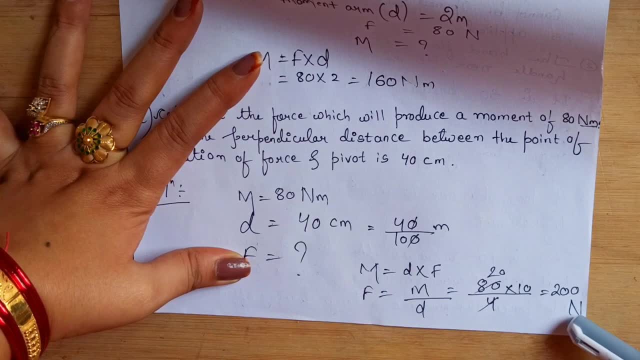 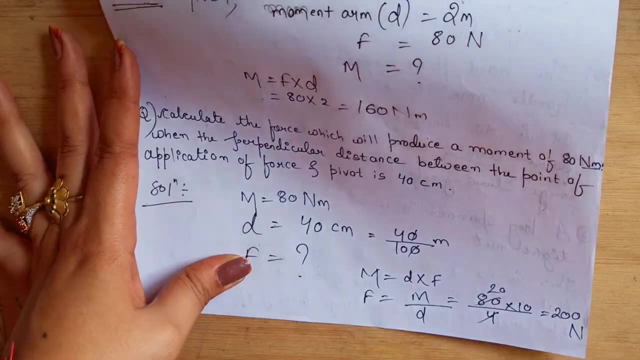 then the answer will be 200 and this is force. so with this newton will go. this is the unit I remember, so I wrote. you must also know how newton came. unit of force is equal to newton. if we do it with dine, then we write. 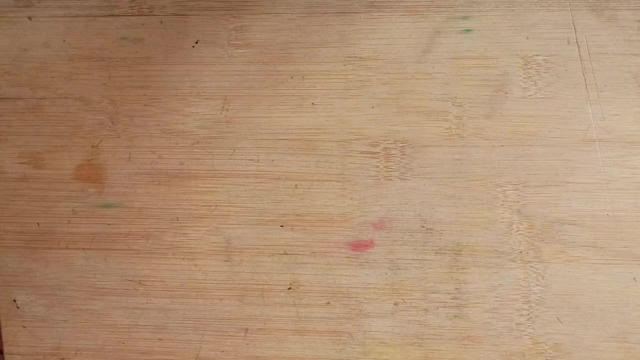 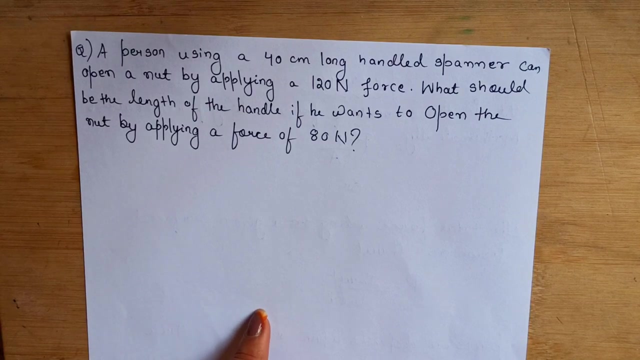 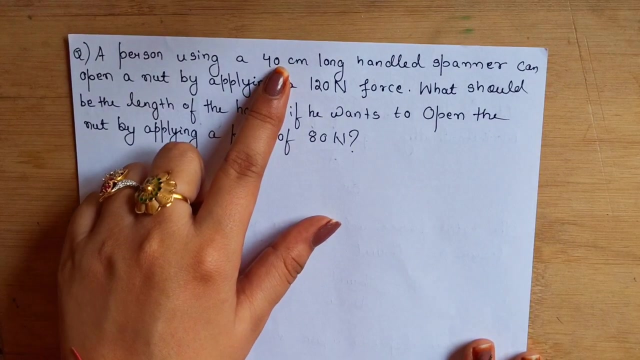 dine. if everything is in CGS, then we write it as it is now. see, this is the last numerical here it is. a person using a 40 cm long handle spanner can open a nut by applying a 120 newton force. now here, 2 things are given. 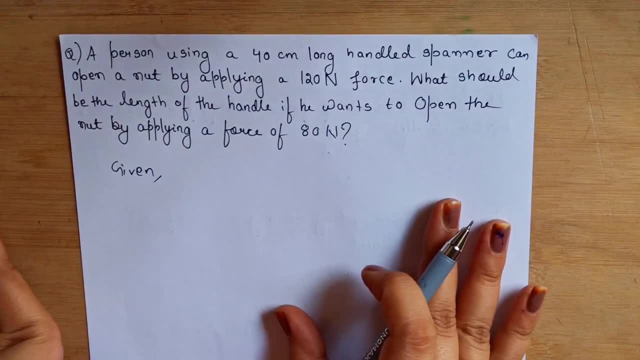 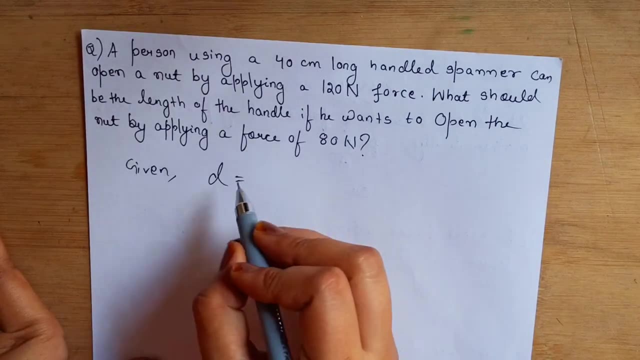 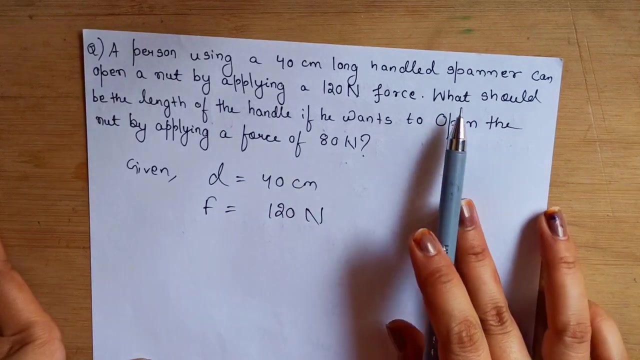 this is distance, momentum, and this is force. first of all movement arm, because this is a long spanner, so this is a long distance, so this is 40 cm. then force is given, how much 120 newton, it is said what should be the length of the handle. 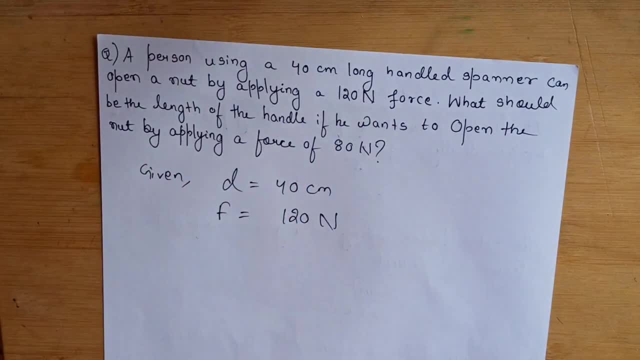 if he wants to open the nut by applying a force of 80 newton means suppose he has a spanner which is 40 cm long and with that 40 cm long spanner he means if he wants to open a nut then he is applying. 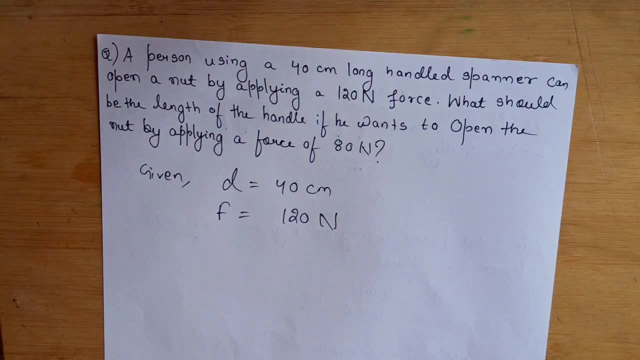 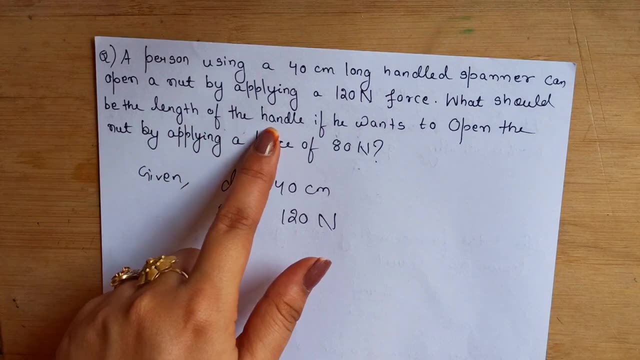 a force of 120 newton. how much 120 newton then? in the second case he is saying that if he wants to open a nut by applying a force of 80 newton, then how much length should be of the spanner? so, no problem. 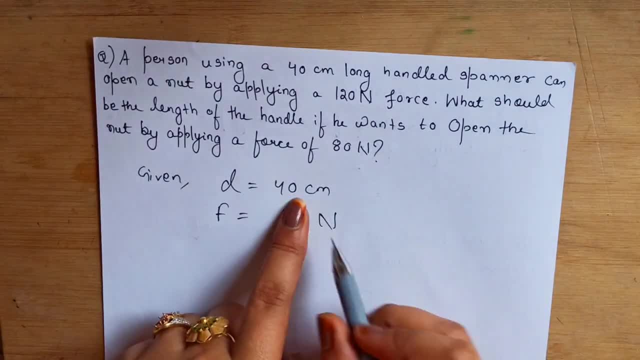 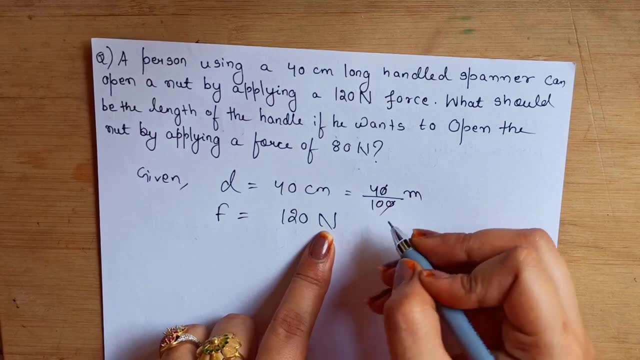 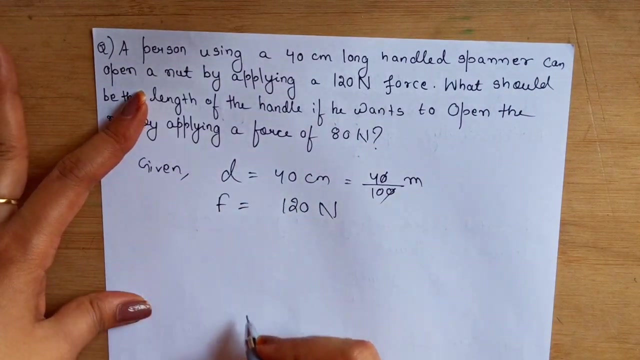 2 conditions are given. so first we will take this condition you will mention here. compare: this is given in newton, this is given in cm. so you guys will do this unit and to convert cm into meter we will divide by 100. ok, now here d is given. 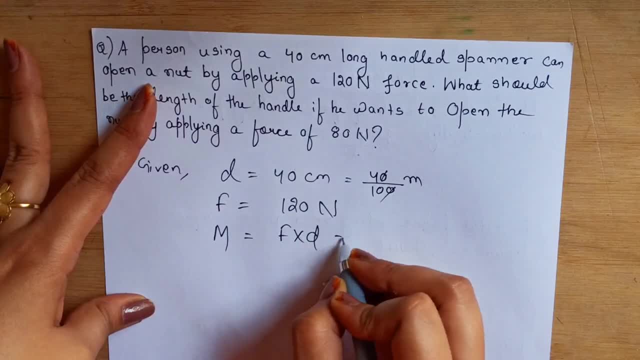 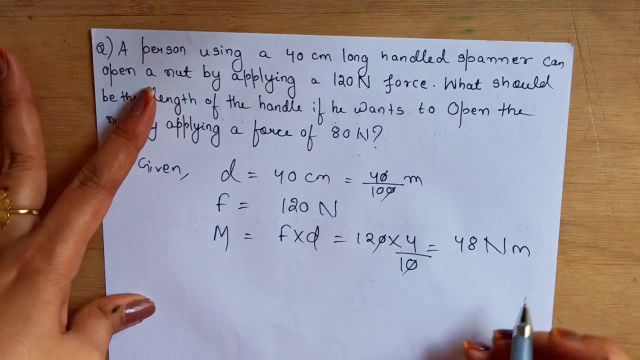 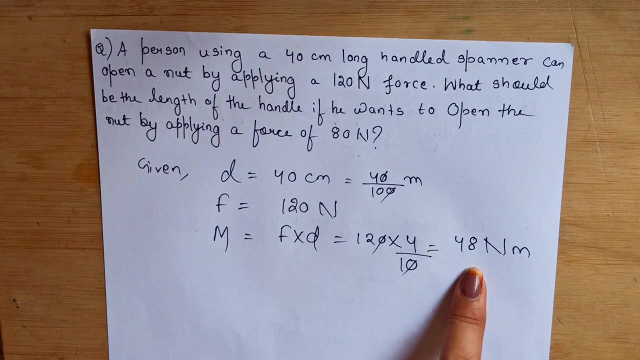 f is given, we will do one thing. we will take moment of force. so f into d, this will be 120 into 4, by 10, 0, 0 cut 12, 4, 0, 48 newton meter means here. in this condition we 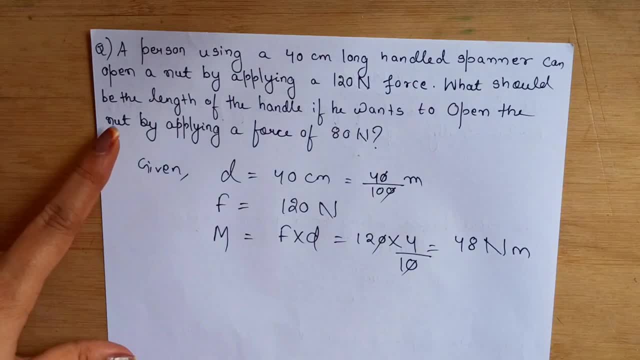 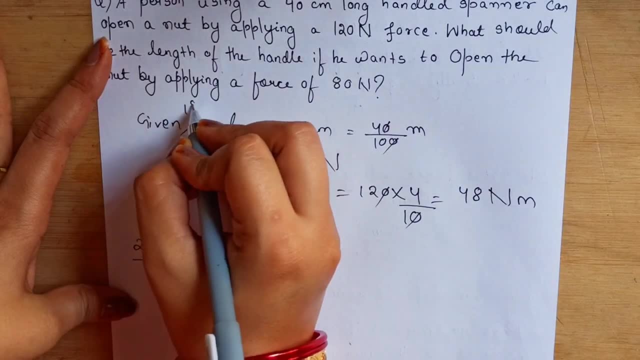 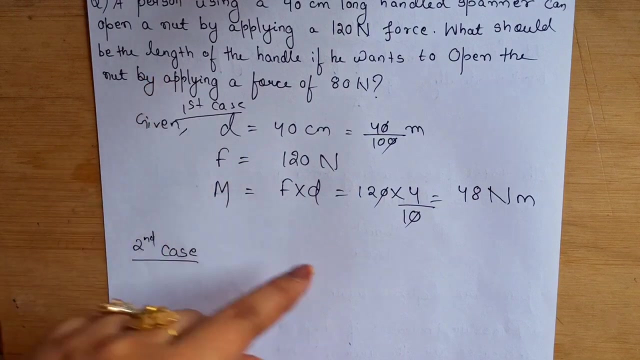 48 newton meter. moment of force is 48 newton meter. in second case what it is saying: that in second case, here I write second case and here I write first case. you can write no problem. in second case what it is saying, that he has to. 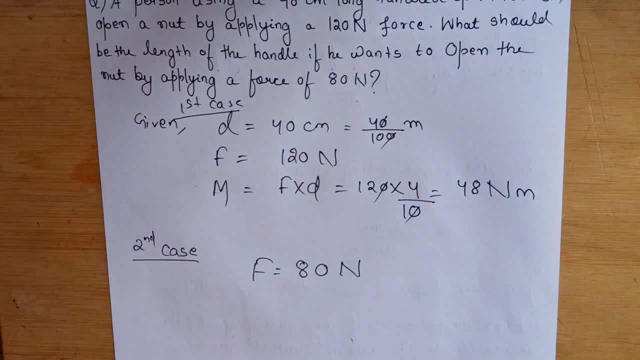 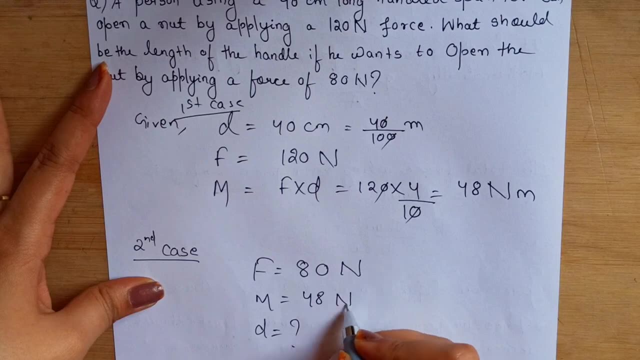 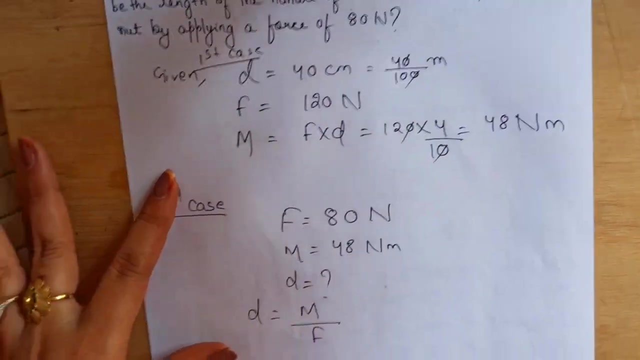 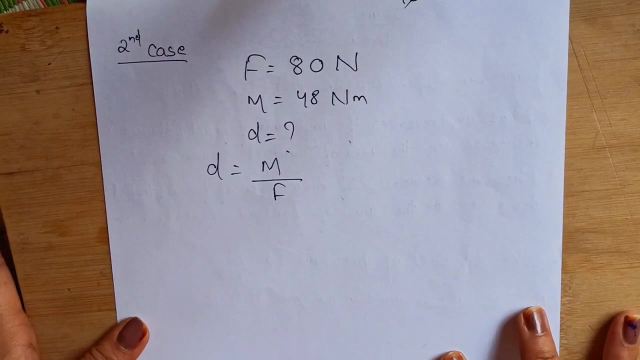 open the same nut and apply that force of 80 newton. ok, so how much length of force is 48 newton meter. so here you have to do d. so if you solve d then the formula will be m by f. I hope you can see. 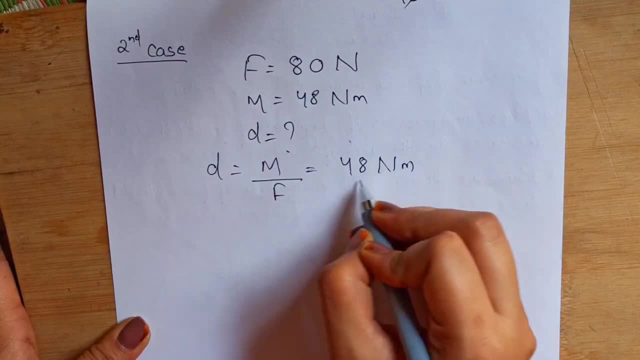 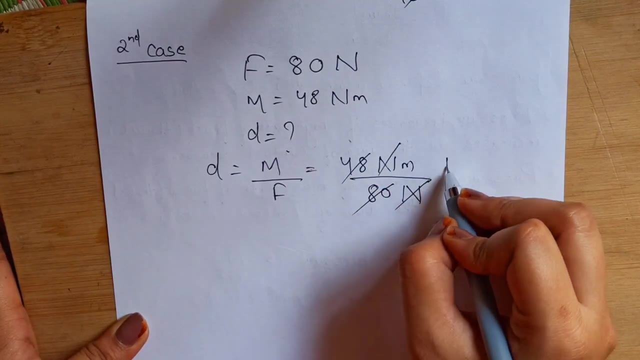 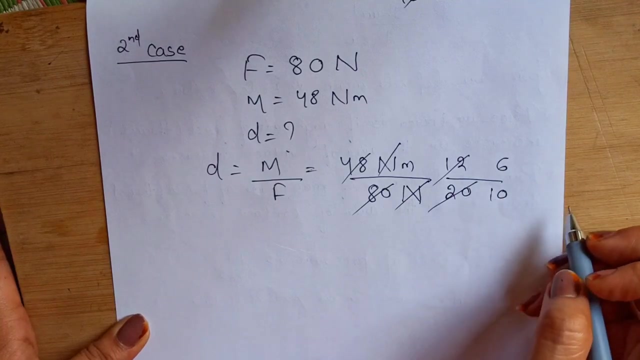 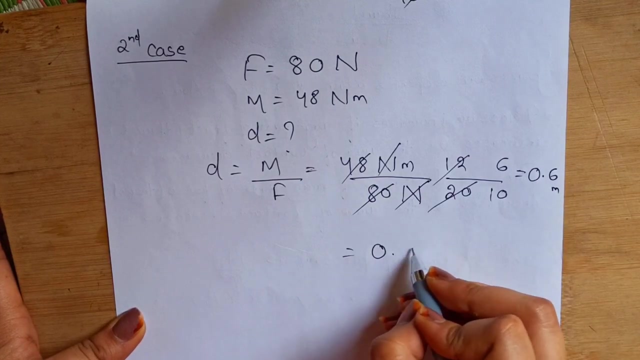 ok, so if you have to take out d, then the formula will be: m by f, m is 48 newton meter. ok, so if you take out d, then the formula will be 0.6 meter. I will make it meter. the answer is 0.6. 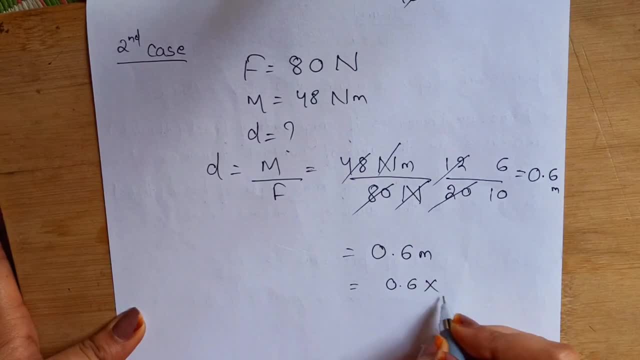 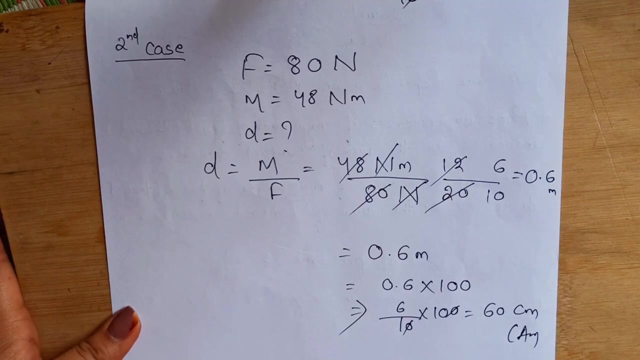 meter. if I want to convert it in centimeters, then to convert in centimeters into 100, so it will be 6, by 10 into 100, so it will be 60 centimeters. this is correct. ok, so I made it the Lorehand регge. 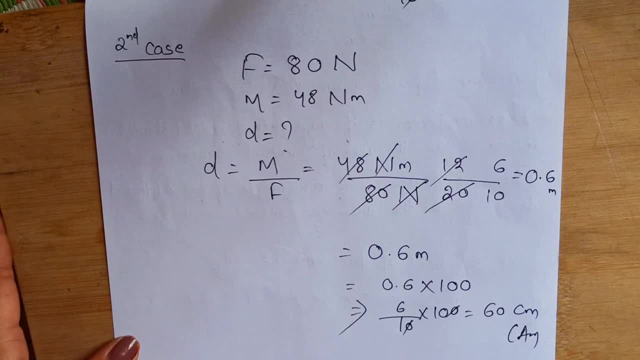 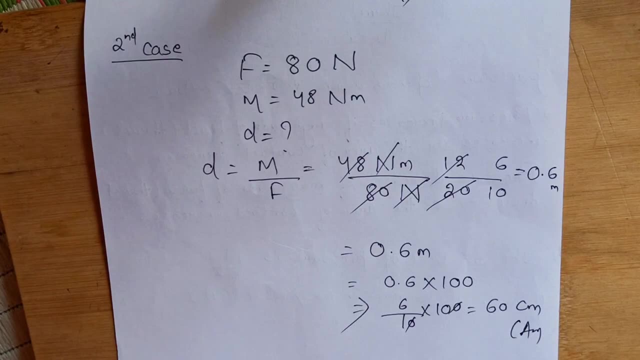 because of this distance length. now you will also finish. now i will help all of you. ok, then, how much you can perform? this will help. how much it needs here. give a and increasing, decreasing pressure, manometer, liquid pressure. there's a lot of things kids. 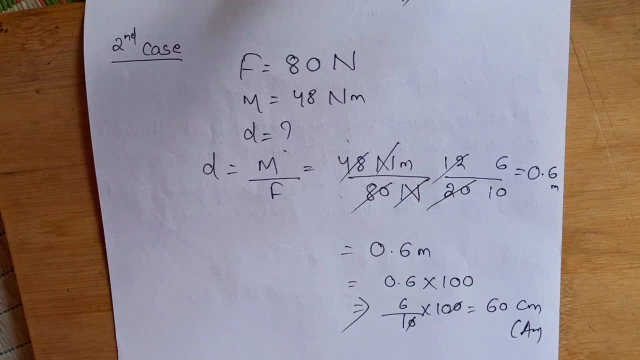 So if you have any doubts, feel free to ask in the comment section, And if you liked the video, then do like, share and subscribe. Thank you.